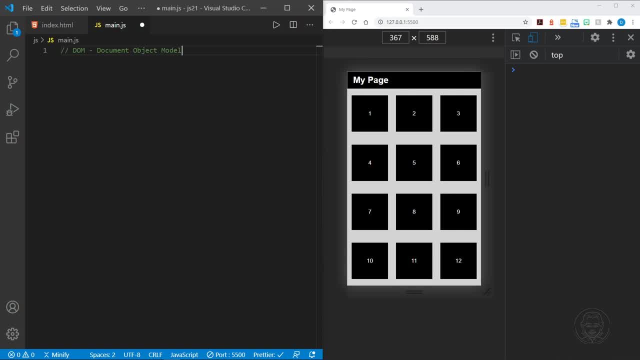 And notice the second word, object. We've already covered objects in our JavaScript playlist and the Document Object Model responds much like you would expect an object to, with both properties and methods. The first thing we're really going to look at are some methods, because we want to select elements. 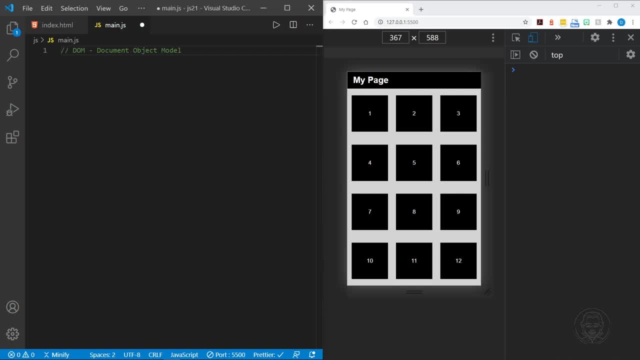 in the document. Now, the Document Object Model was not just designed for HTML, but in this regard, we will be looking at HTML pages, so specifically the HTML DOM, And let's discuss how we select an element with an ID first. You can see I have a web page open. 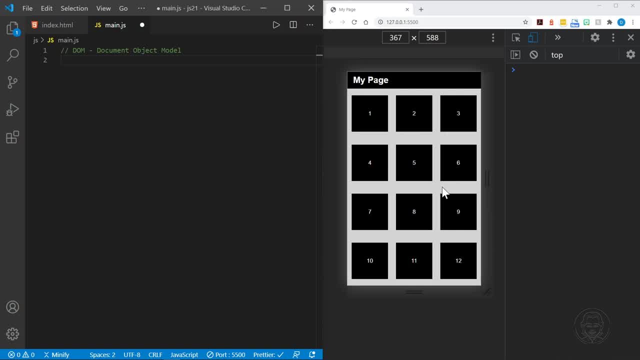 and on this page I have 12 identical divs and I'm using Flexbox for these divs, so if I scrunch the page, of course they flex and I could widen it out even further and it would go to four or more per line as well. 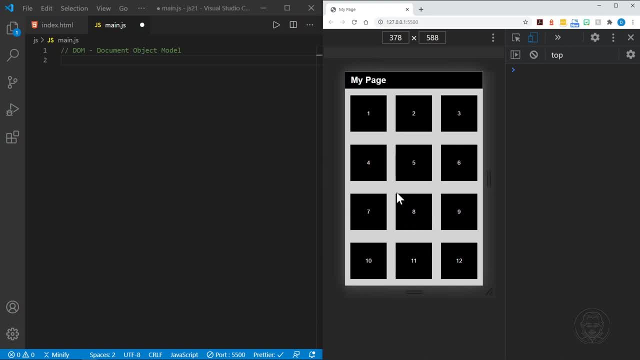 It's a totally flexible design for responsive design as far as that goes, and I've got the console way over here on the far right as well. So I'm going to write some code and the first one is to select the first div. 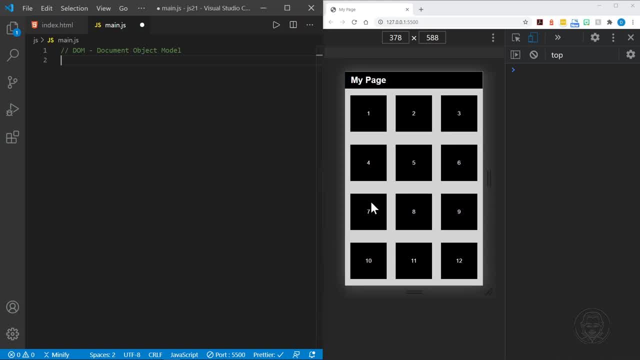 because I've actually created two views. so this view you see here is a section that has these 12 divs, and I'm going to define the first view in a variable called View1, and I'm going to select that view with DocumentGetElementById. 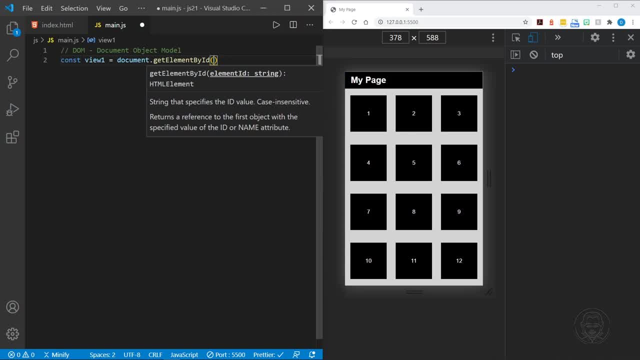 and, of course, we only give a specific ID to one element in our web page, and I will choose View1, because that is the ID I gave this first view. Now, if I log to the console View1,, we should see that element returned. 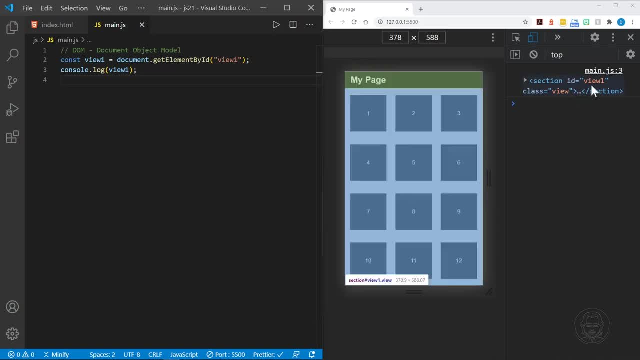 and that's what we see over here. We've got a section and it has View1 ID and it also has a class View and you can see in the page. as soon as I highlight that in the console, it highlights the page, since I have the dev tools open. 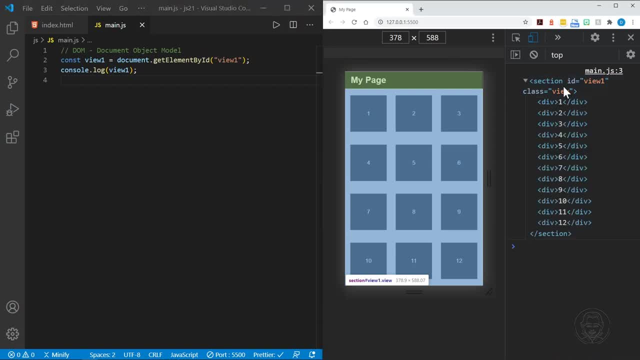 And we can break down the section by clicking the arrow and then it shows all 12 divs and it will highlight each one of those as I mouse over them, And that's much like you would expect properties to do if we had a class when we click the arrow. 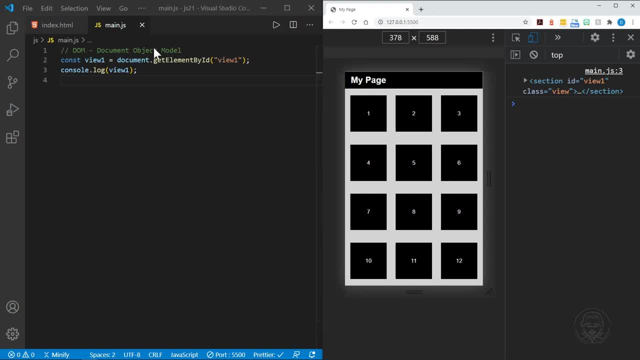 and it would show the individual properties of a class. So that is how we select an element by the ID. Now let's go ahead and look at another way to do that, Possibly a more popular way, as I see many using this: the query selector. 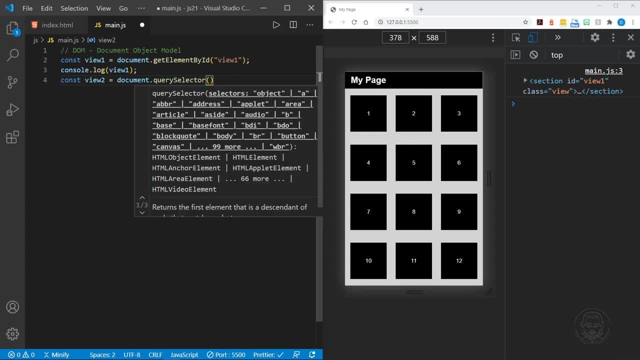 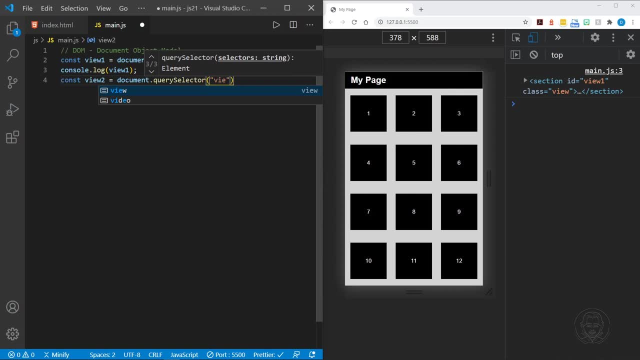 With the query selector. it's not just meant to select elements by their ID, It can select by other methods or by other means. So when we do this we can't just say View2, because we have the second view, or View1.. 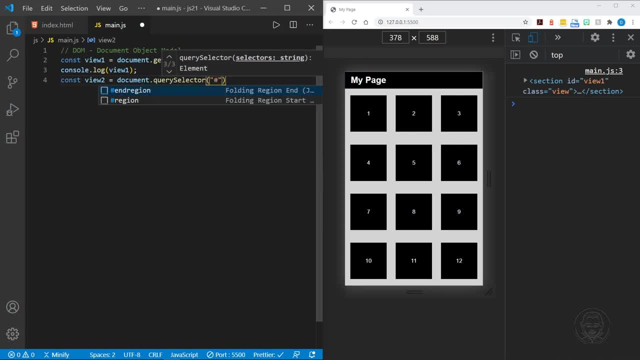 We'd have to use the hashtag or pound symbol to indicate that it's an ID. So that is a main difference between the get element by ID selector and the query selector. So now I'm selecting the second view and I'll log it to the console as well. 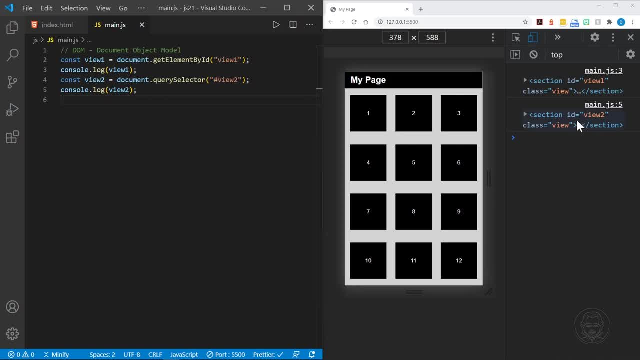 I save our page. Now you can see we get the second view and it's not highlighted because it's not even showing over here on the page yet. But it has an ID attribute and it has a class attribute And if we open it up it doesn't have all the divs. 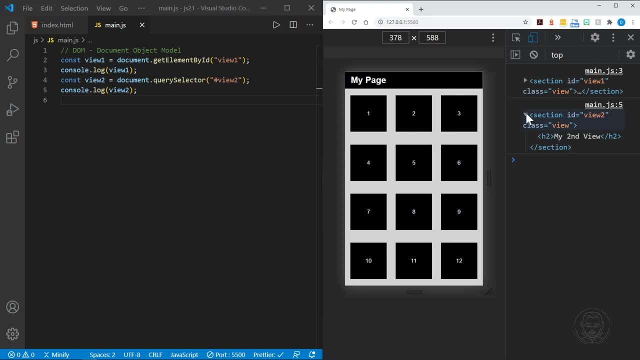 It just has an H2 element inside of it saying my second view, And so there's two different ways, of course, to select by ID, and we just displayed both of those. Now let's look at changing the style to actually show or hide the different views we have. 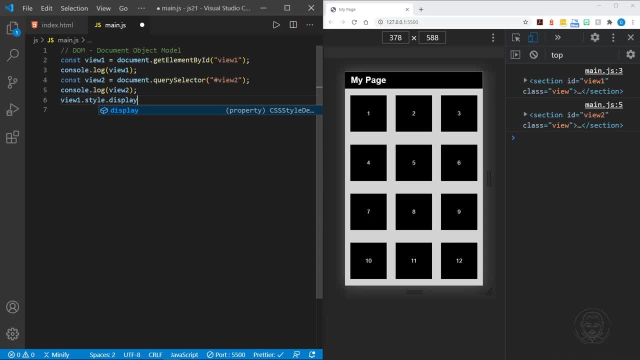 So this is how you could have a single page application or a spa that could actually have more than one view, because you can hide the different views. In this case, at the top I have a nav element. It will always show, but underneath that, 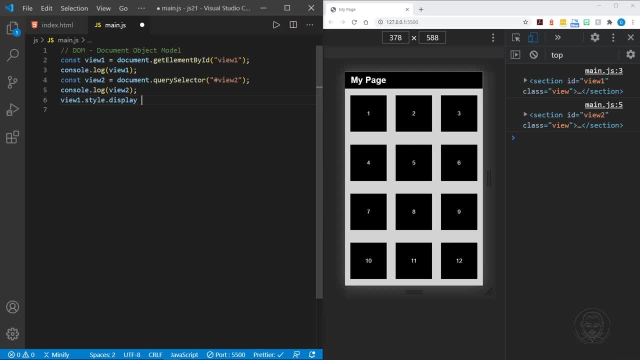 I have sections and we can show and hide those. So I've got the display for view one and I'm going to set it to none And then, for view two, set the display And notice we're actually changing the CSS properties here. 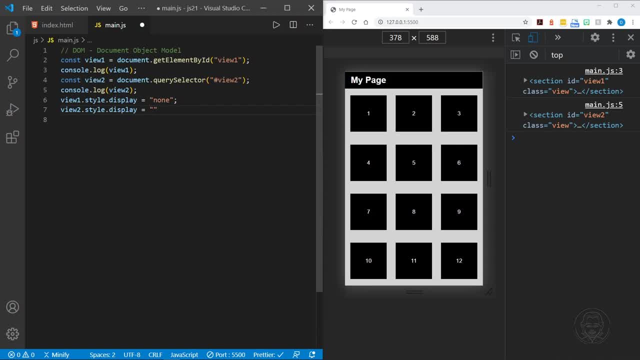 by accessing the style property and then the display property of the style property, And I'm going to set it to five, I'm going to set it to flex and now we'll save our page And you can see, we see the second view. 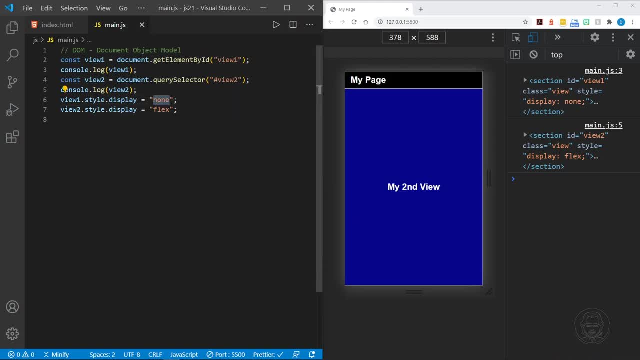 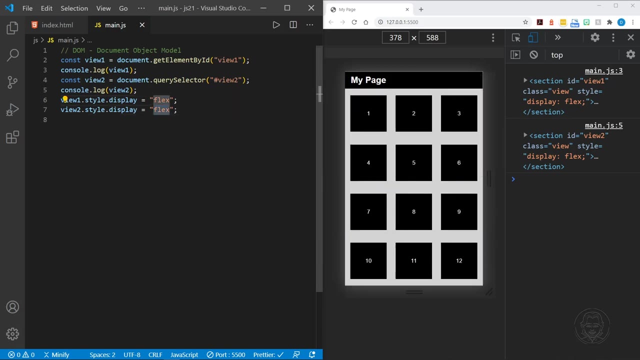 and the first view is no longer displayed. And if I change that and I set both to flex, now we've got the first view and I can scroll and actually show you the second view. Before that I couldn't scroll. So if I set the second one to none, 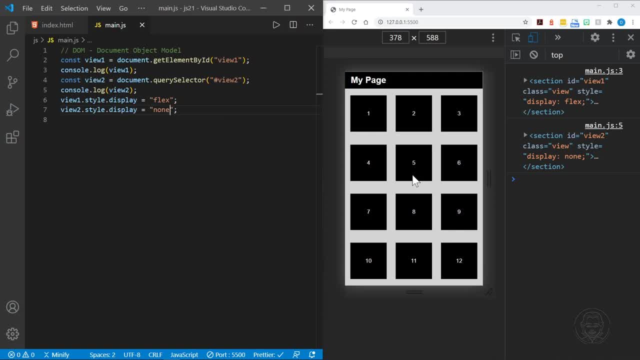 now there's no scrolling. This is what is available and we could toggle between the two, or we could have more views and we could show and hide those with a method or function we create, and that would help us have a single page application. 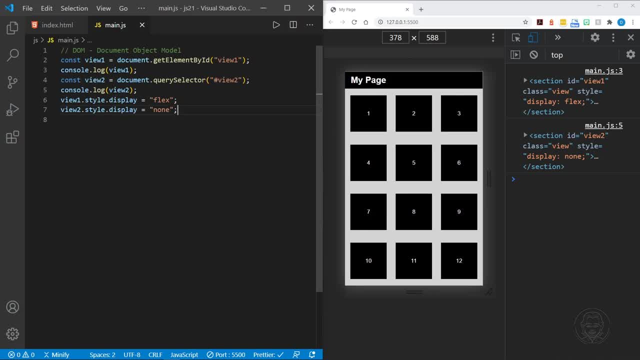 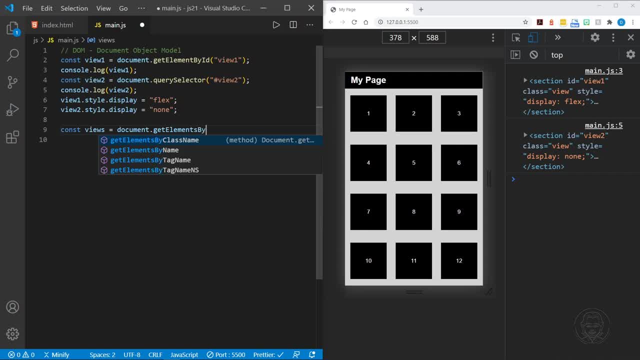 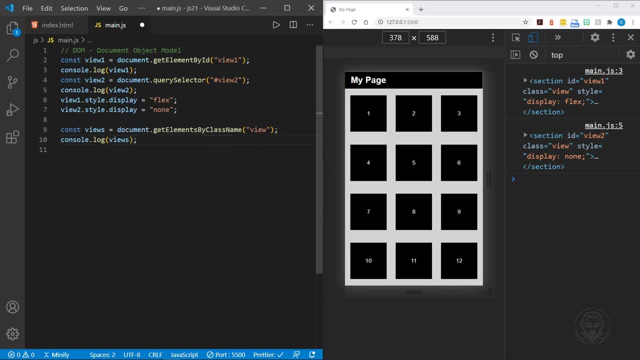 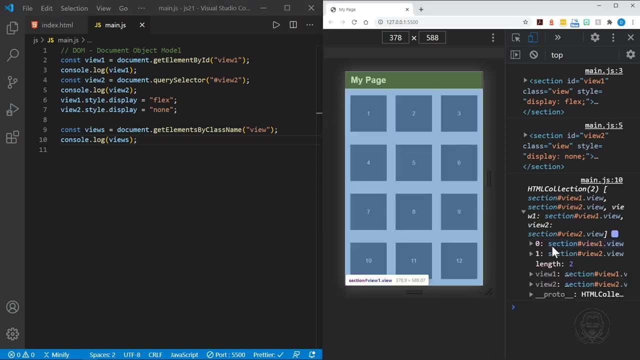 and we'll log this to the console and you can see what is returned. We get an HTML collection which is like an array, but it's not exactly an array, And inside this collection there are there are two items, two elements. 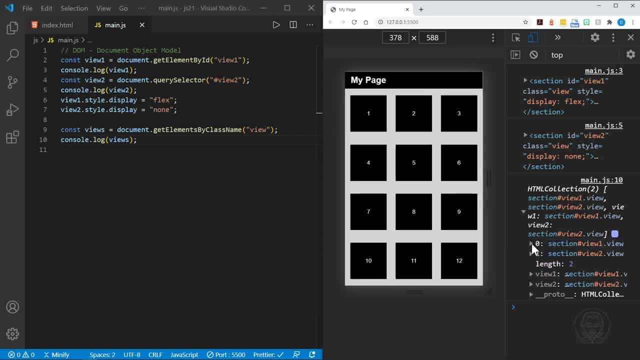 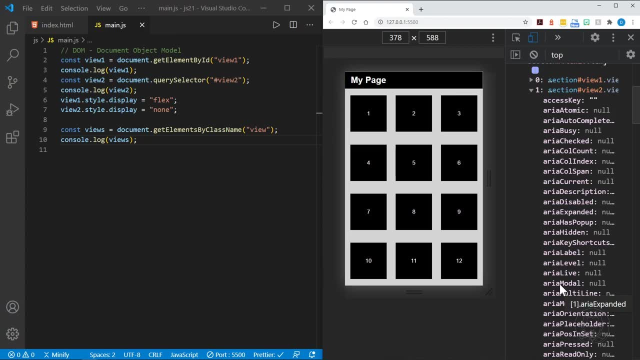 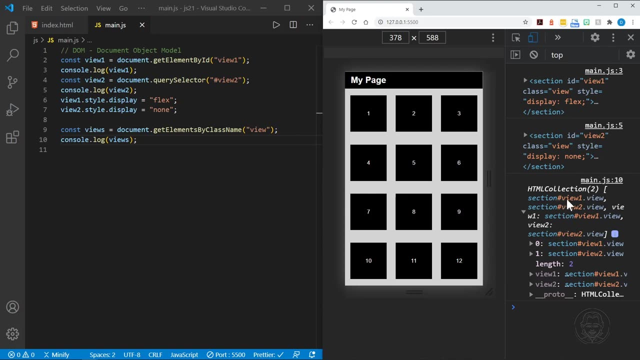 and we see the first and the second one. I'm highlighting the first view here, and then there's the second view. You see all these different possibilities for properties. Most of them are null for this section. Notice also that it shows the ID. 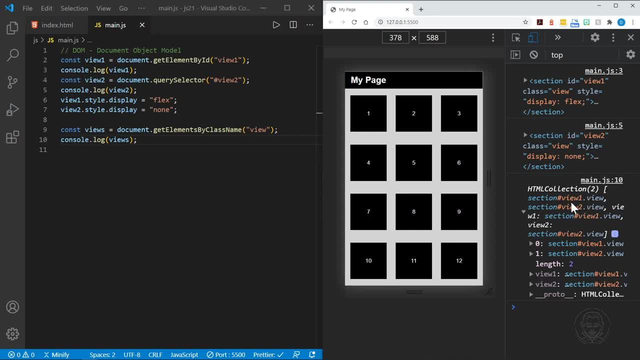 and then the dot in the class. This is how they will display, because they have an ID attribute and then they have the class, And if there was more than one class, it would show each one. It would say dot, view, dot, whatever the next class is. 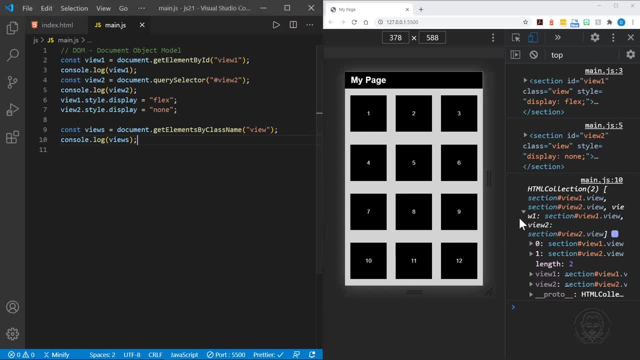 and so on. So there we have an HTML collection with two elements inside of it. Let's look at another way to select the views. So I'll say const sameViews and I'll say documentquerySelector again. but this is different, We'll say all. 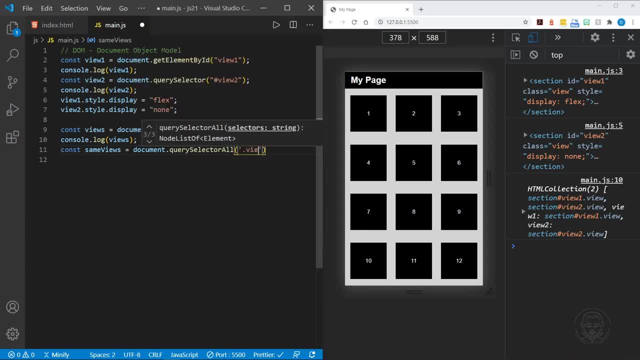 Now we expect more than one. We're going to select the classes. So once again, with the querySelector, we have to specify that it's a class, just like we would in CSS with the period And just like we did up here with the querySelector. 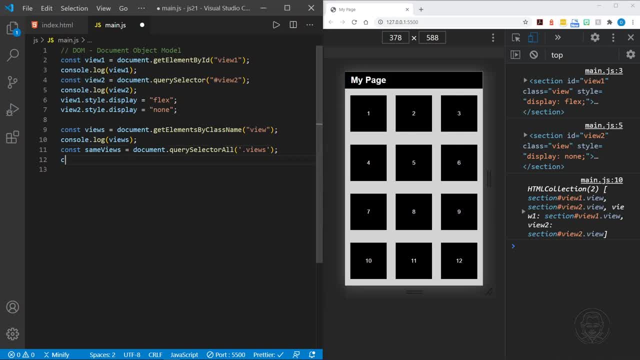 for an ID, we had to use the hashtag, And now we'll log that to the console And with sameViews we get a nodeList. And what did I do wrong? There is some reason. our nodeList has no items at this point. 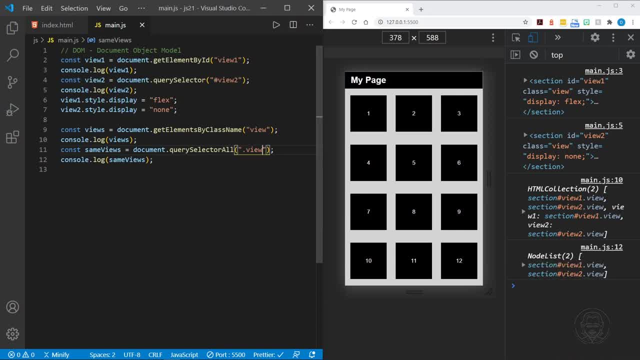 Oh, I said views. There we go. It's just view class. I was thinking views. Now our nodeList has two elements. There they both are. Notice the difference in HTML collection and a nodeList. What could be different about those? HTML collection actually has elements inside of it. 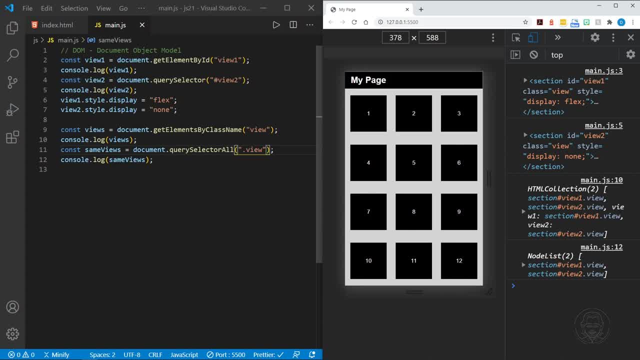 A nodeList has nodes and in the HTML DOM nodes are everything. Nodes are white space. Nodes can be simply text inside of an element. So there are more nodes than there are elements in a webpage And the HTML DOM recognizes all of those nodes. 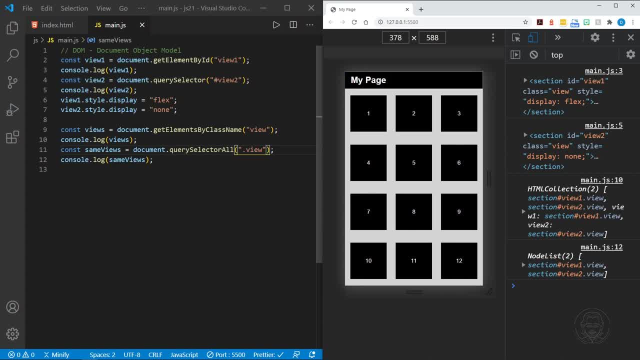 So we do have to be aware of the difference between a node and an HTML element. OK, So that is how we select: by className. We've looked at Git, element by ID and gitElements by className. We've looked at the querySelector and the querySelectorAll and I'm sure 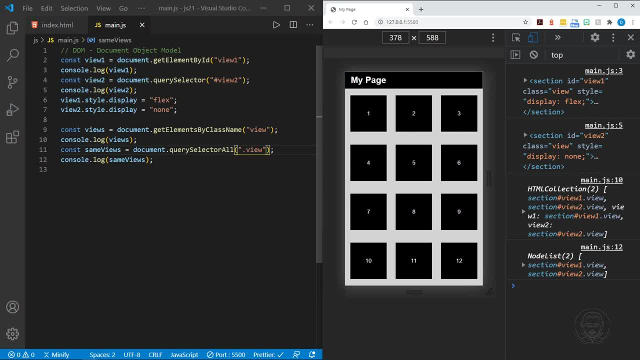 sure you're gathering that the query selector uses selectors, much like our CSS does, to identify the different elements on the page. Now let's look at these individual divs in our first view. So I'm going to define divs and I'll set that equal to view1 and then put my selector after that. So then I'll put: 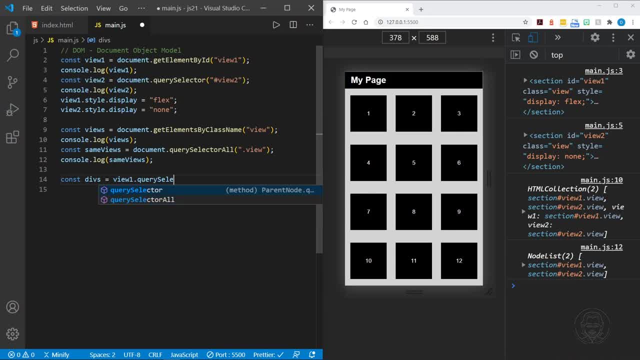 query selector, all, and I'm going to select the div and notice I don't have to put a hashtag or a period or anything. I am just selecting the actual tag name here, but I am starting it out with essentially the results from a previous query. I don't have to say document, I'm just looking within the first view that. 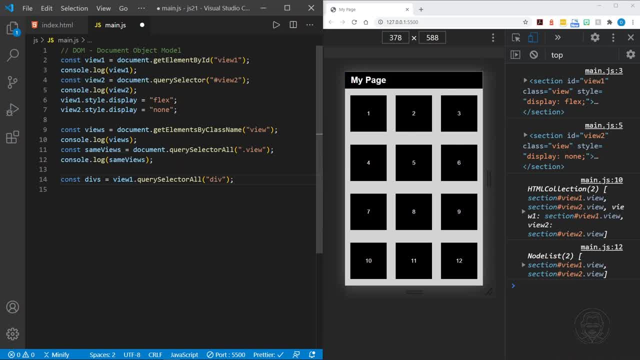 I've already selected. So I'm starting the selector out with view1, then using dot notation and saying query selector all and selecting all of the divs specifically within view1.. So now I will log those and you can see we get a node list with 12 divs. Now let's get the same divs in a. 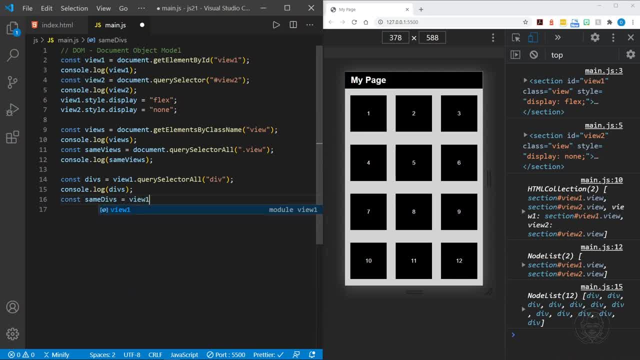 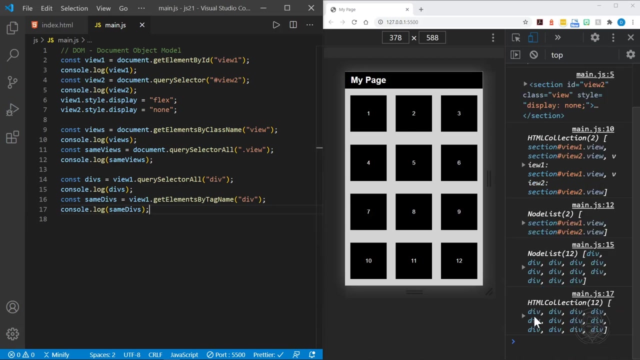 different way. Say: view1 dot. get elements by tag name. This is another version of get elements. If I log those, you'll see we get an HTML collection with 12 divs. Let me go ahead and open this up Now. as I highlight the divs, you'll see them highlight on the. 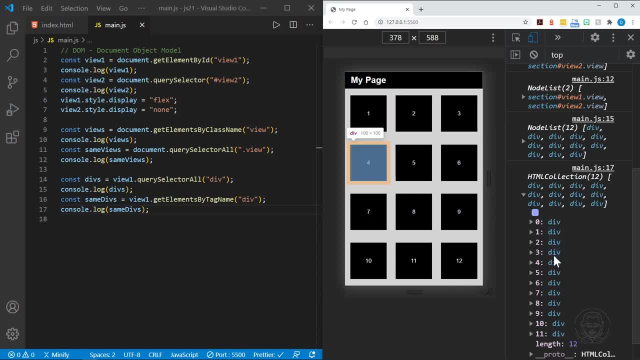 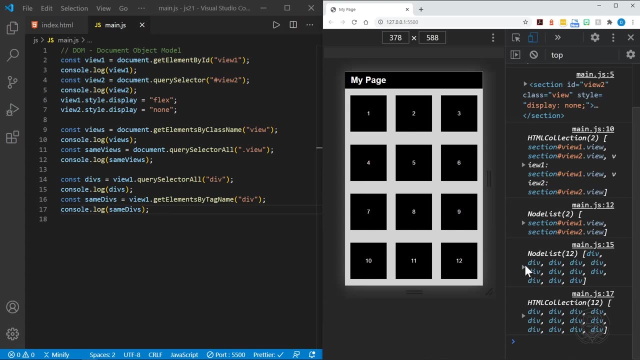 web page and just mouse over each one and they light up, so we know which one we're looking at, And then they have all of the properties within them, just like you would expect from an object. So there are all the divs in the HTML collection. We can do the same with the node list. 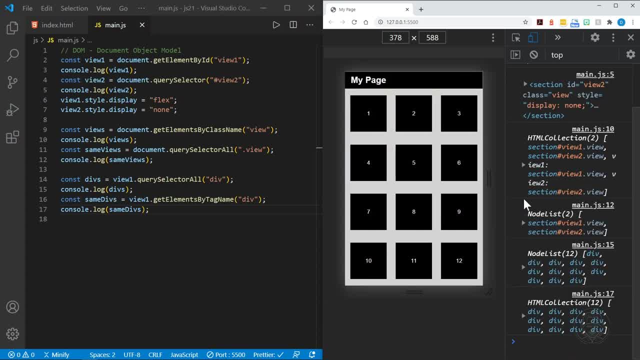 actually, and they all highlight when we do that as well. Okay, so now we have selected by tag name and we also built our selector on a previous selector, So that really helps us out. Now let's get a little more specific with selectors. So say, we just want to select the even. 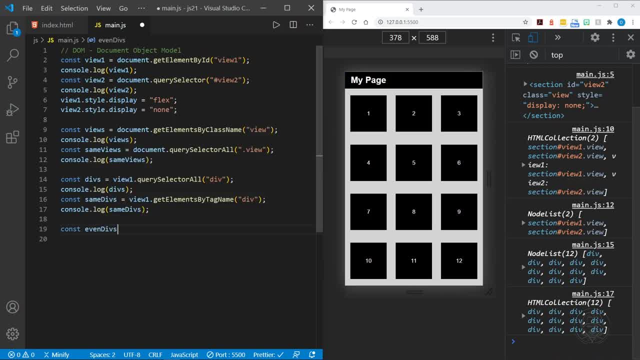 divs out of these 12.. So we just want 2,, 4, 6 and so on. I'll start with view1 once again, because all the divs are within view1.. Say, query, selector, all, and now we get more specific, just like we would within CSS. So I specify div, then 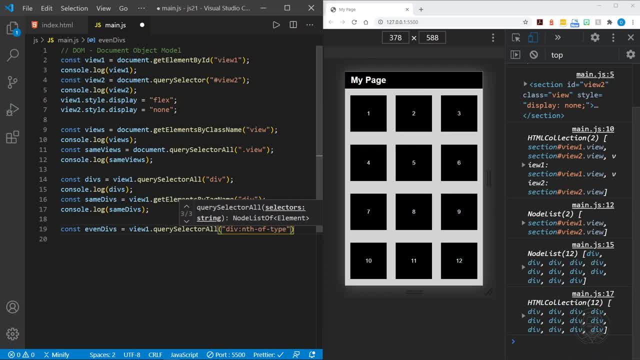 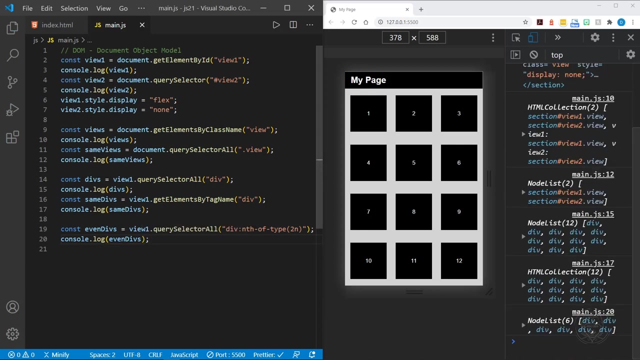 I'm going to use nth of type And I want just the even divs, So I provide that extra information there with the 2n, and that's what I need. Now I need to log this to the console. Notice we get a node list back, as we'd expect, with query selector, all And it. 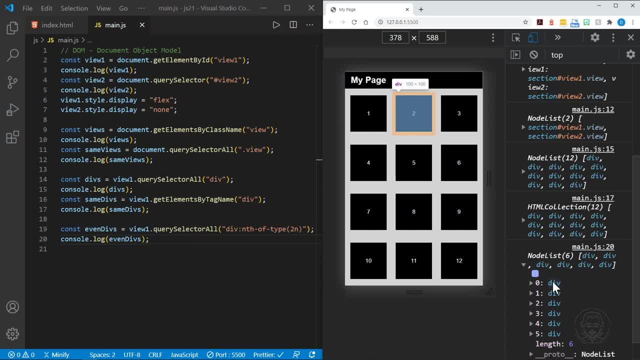 has six divs. Now we can highlight those, and the first one is the last div Bye, the first even div It's. number two then should go to number four, number six, number eight, 10, and 12.. 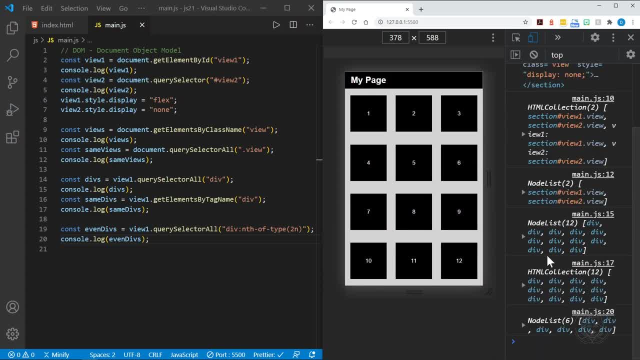 We selected just the even divs within our page, And that is by knowing how to use our query selector. And, essentially, if you know how to do that in CSS, you know how to do that within the query selectors as well. Now, what if we wanted to actually alter our page? 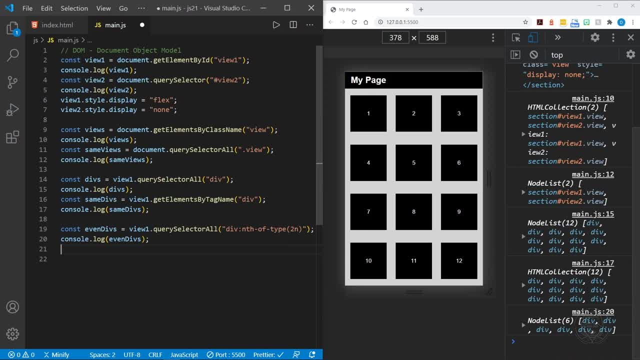 We're selecting these. so what do we do with them? You know we did change the display property- We had flex or none- to either display our flexbox layout or to hide the views we don't wanna see. So we did alter our document in that regard. 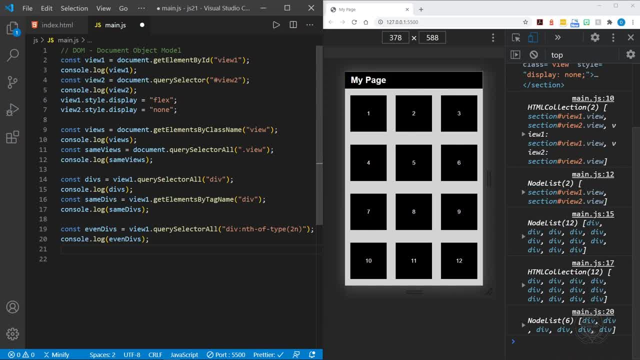 There's, you can really change just about anything you want to. So let's do something else. We'll say: just like an array, we'll use a function, we'll use a for loop to work our way through these even divs. 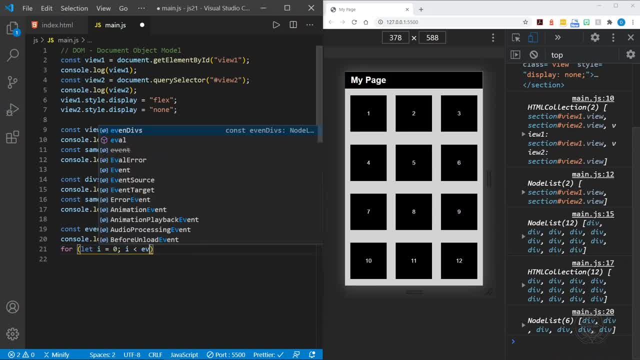 We'll say: while i is less than even divs dot length, and then we'll up our increment variable. there we go. So there's our for loop, And now we'll programmatically select each of the even divs as the loop goes through. 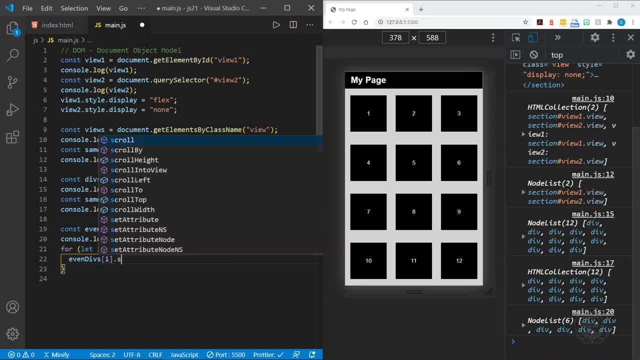 with using the iterator there And we'll say style. And then let's change the background color of our even divs And let's set it equal to dark blue. That should stand out And we don't really need to do anything else. 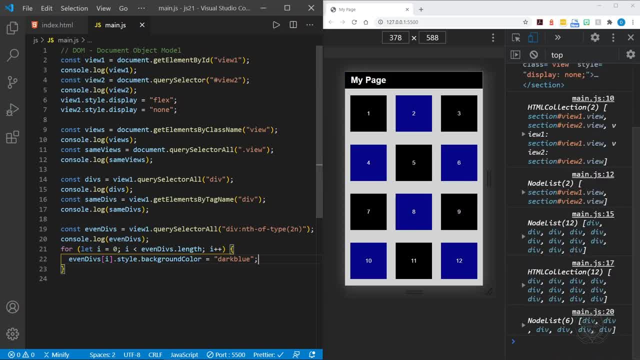 I think that'll do the work for us. We'll save that And look at that. we've changed the background color to each one of the even divs in the view, in view one, And we could do other things as well. 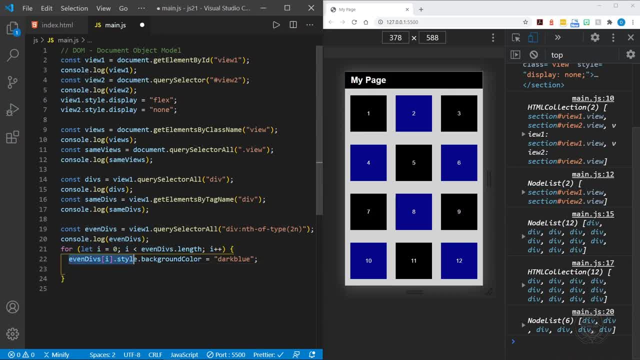 So we could do this same, even divs, dot style, and then we could refer to say the width, And these divs are 100 pixels by 100 pixels, so just 100 pixel squares. Let's set the width equal to 200 pixels. 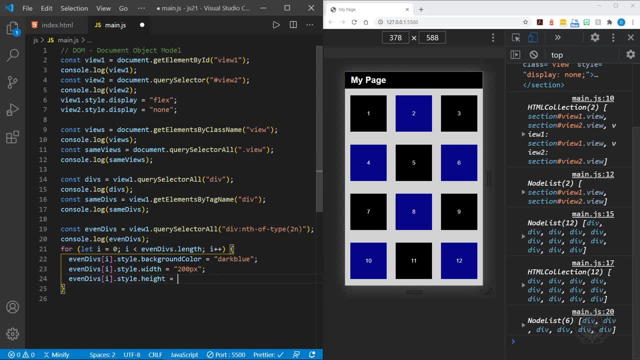 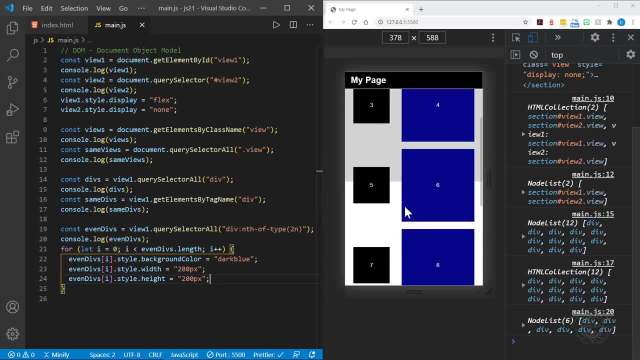 And let's do the same to the height. We save that and, wow, that changed our layout dramatically, didn't it? So we can squeeze that in Single column. I don't quite have enough room to squeeze it out. Let me see if we can just widen this out a little bit. 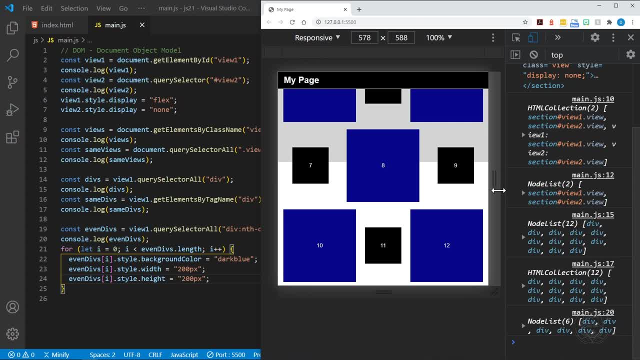 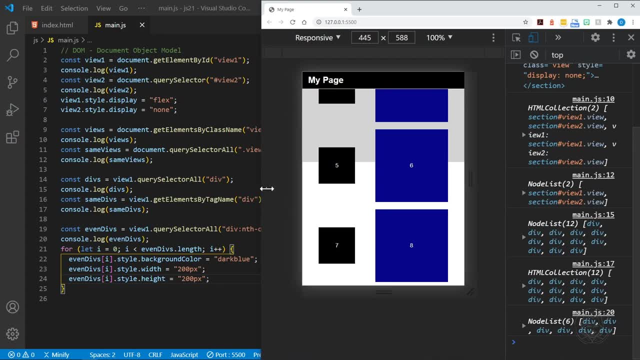 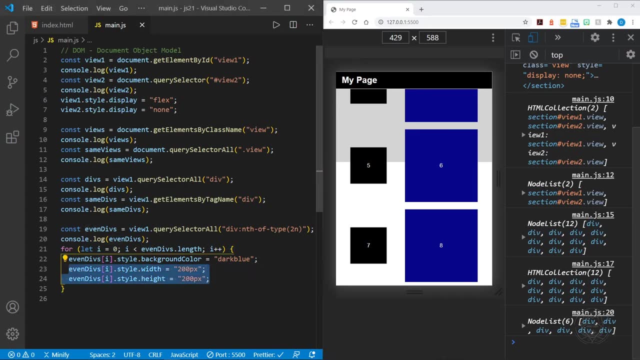 to see what it would look like. There we go. Definitely looks interesting. We may not want to keep that, but we'll take a look at it. at least Got that back to where it was. so I'll comment these out to get our even grid back. 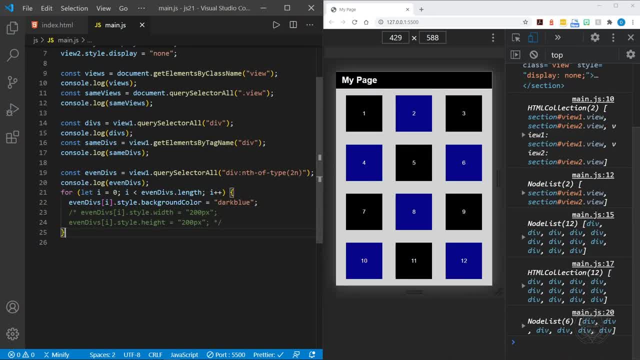 Just an example of how you can do that. You can alter every little bit of the web page that you want to by altering the style, so you're changing the appearance. Let's look at changing, maybe, some text. So now let's look at the nav bar. 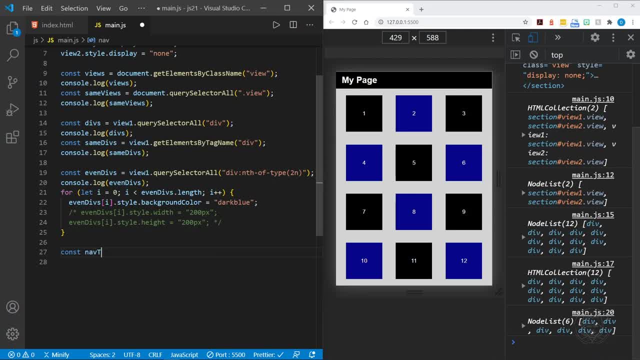 We've got my page up in the nav bar and I'll set this variable equal to nav text and we'll say document dot, query selector, and we're going to choose the nav bar and then that's an H1 element. So 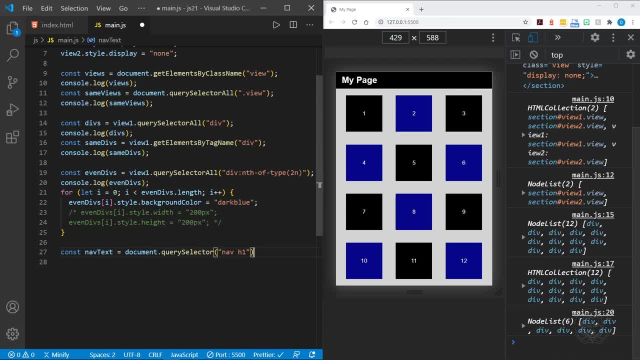 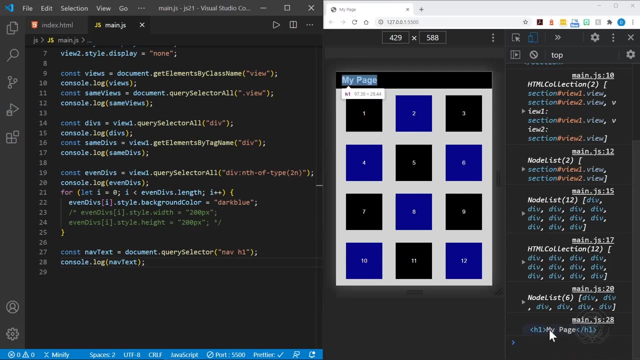 Inside of the nav bar. I want the H1. And now I can log that and we should get our H1 element in the console. That is exactly what we got and as I mouse over that, you can see my page highlighted in the nav bar. 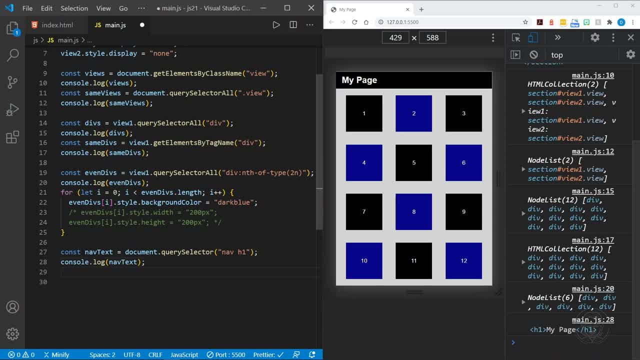 That's our H1.. So now I'll say nav text dot to start our next selection And I'll go to the text selector and we'll choose the text content And we'll change the text in that and we'll say hello world. 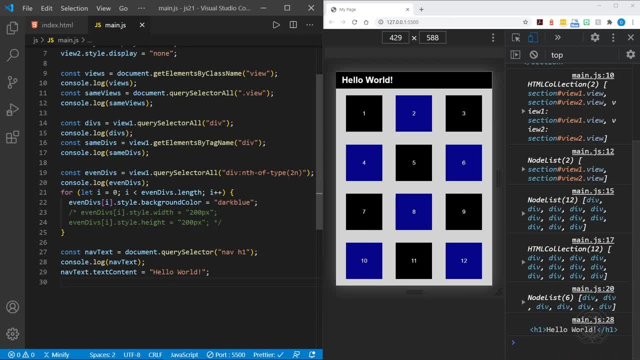 You save that and my page changes to hello world at the top of the page. And since we logged that, we got hello world right away as well, even though the log was above. That's just a little bit of a bonus, Interesting, huh. 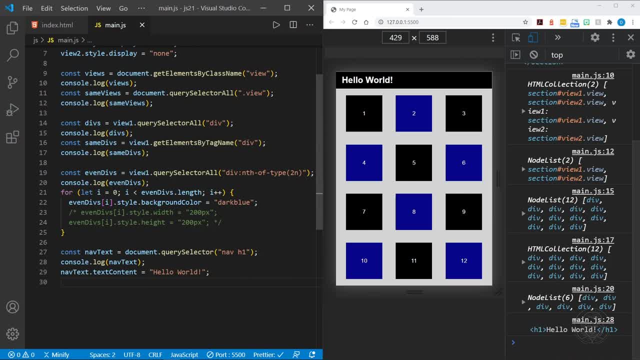 Okay, Next let's define our nav bar itself. Let's say, document dot, query selector. And now we're just selecting the nav. So that's just the nav bar. And now, with this nav bar, we can change the inner HTML. 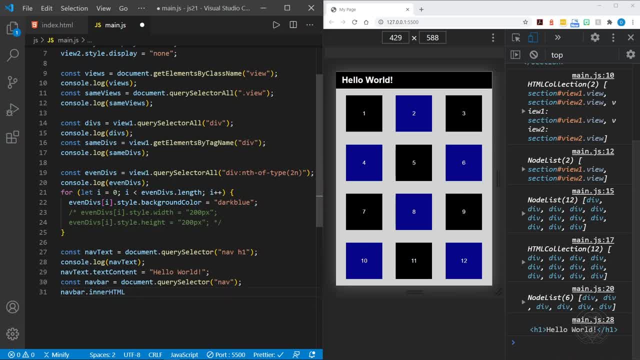 Now it is important to know how this is different from text content before we just change the text. So that is really the text node that we're changing and it is not adding any HTML to the page. However, the inner HTML property will change the HTML. 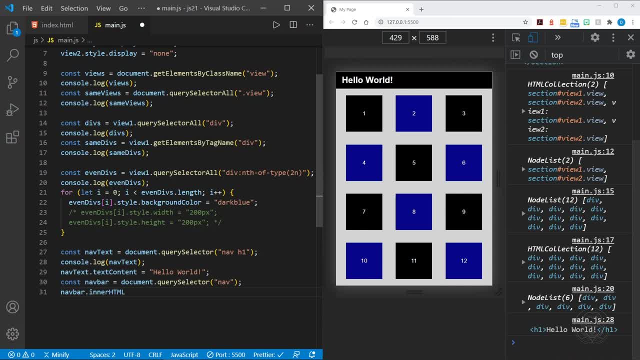 if we insert it, We can actually insert HTML with inner HTML property. So let's do that and we'll add, because the inner HTML, by the way, will overwrite everything that we currently have in there. So we need to put something like our hello world. 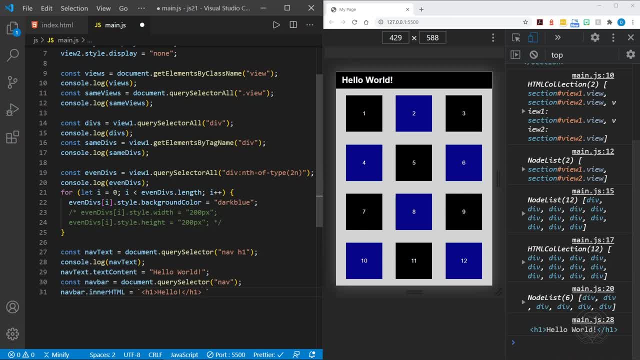 I'll just put hello so we know it's different. And then I'm going to add a space and I'm going to add a paragraph And here in the paragraph I'm going to say: this should align right, And that is because of the flexbox layout. 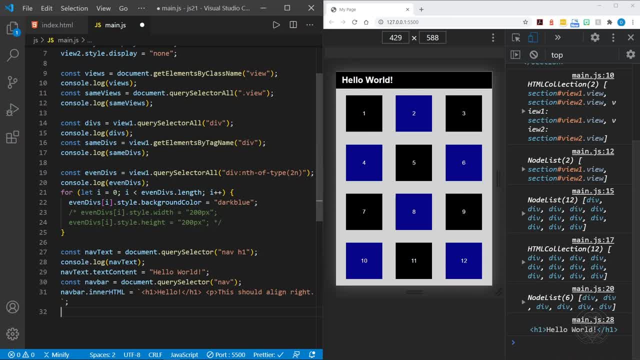 that I have for the nav bar. I am using the justify content with the value set to space between. So we'll take a look at that And after we do this, I'll just save this And you can see that the hello was hello world. 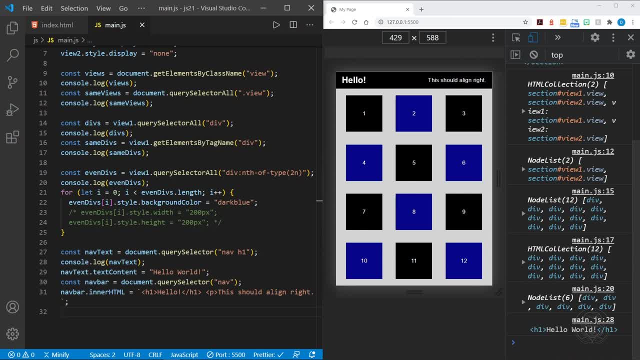 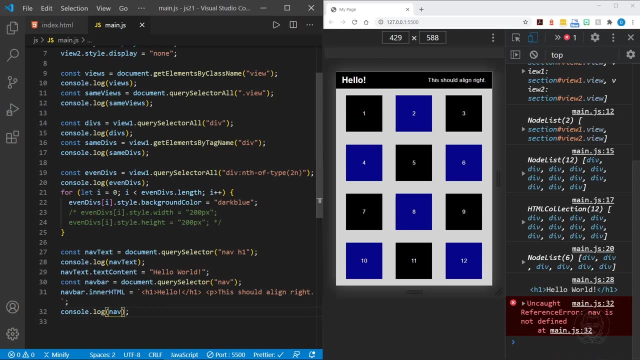 changed to hello and the paragraph that says this should align right is now aligned right. So if we log our nav, nav is not defined. oh, I called it nav bar. There we go, Nav bar, let's log our nav bar. 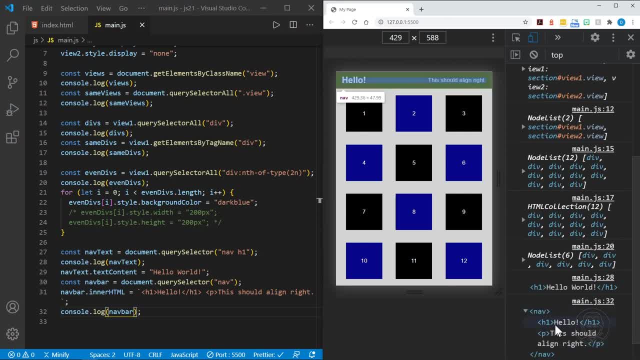 Here it is, Let's break this down. And we've got two elements inside it that we just inserted. We've got our h1 hello and we've got our paragraph that says this should align right Now. what if we wanted to change that alignment? 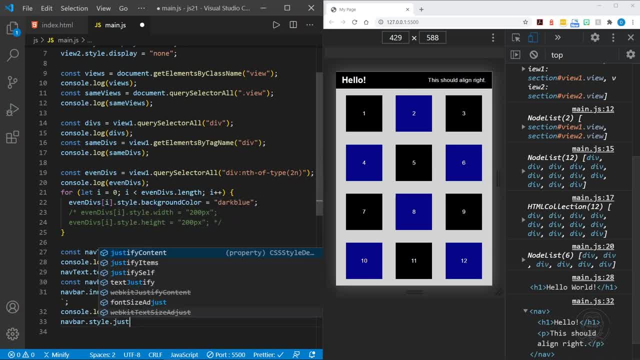 We can also do that by altering the style of the nav bar, And it is a flexbox and I have justified the content. So we can justify the content in several ways, Knowing how or what properties it accepts. So flex start should send everything to the left. 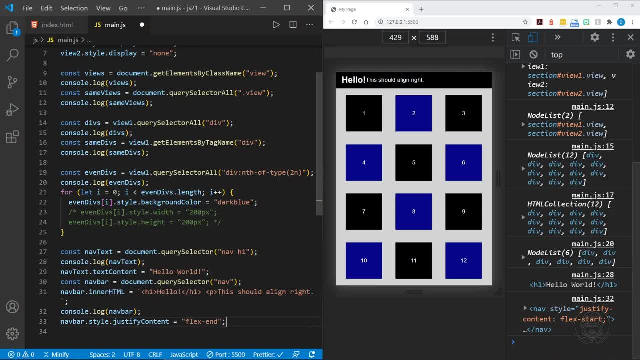 There we go. Flex in should send everything to the right. Sure does. We were using space between. What if we say space evenly? And it spaces it out evenly, of course, from the sides as well. So the reason I like space between: 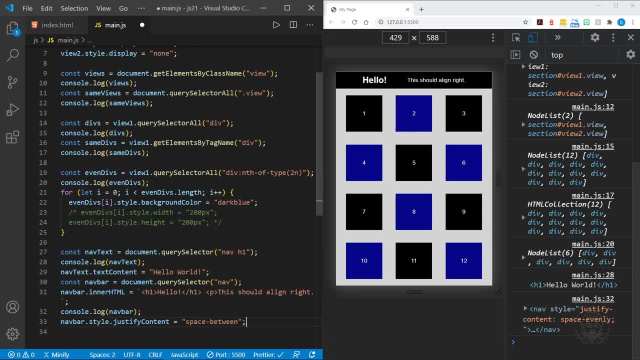 is because it aligned things right and left, which looks kind of good in a nav bar, And you can see that. So we've got hello on the left and this should align right on the right. Now let's talk about navigating the DOM tree. 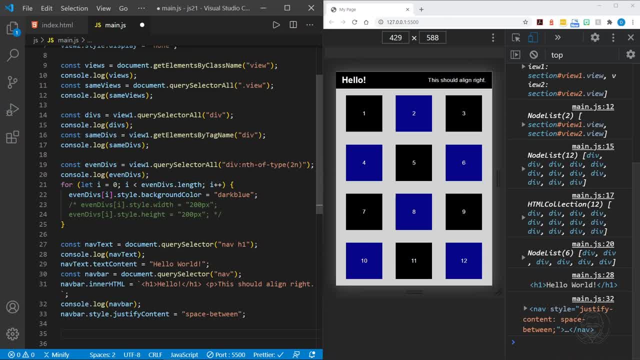 And this gets fairly interesting. You don't have to get too complex with this that many times in your page, but there could come a time where you need it. So remember we have our even divs that I'm going to refer to. 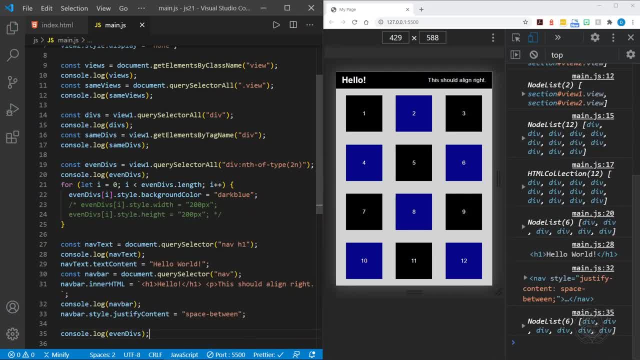 We selected those earlier, So I'll just log that once again to the console. You can see it's a node list with six different nodes in the list, And now, instead of just logging even divs, I'll just log the first one. 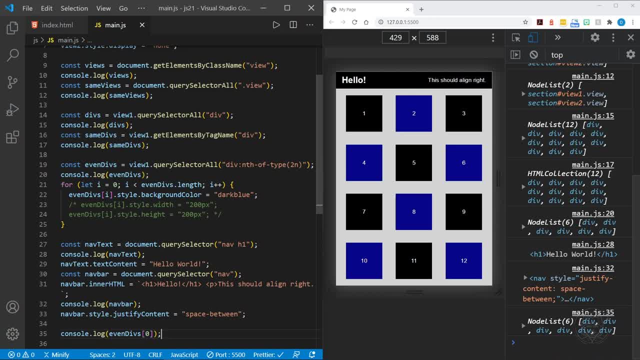 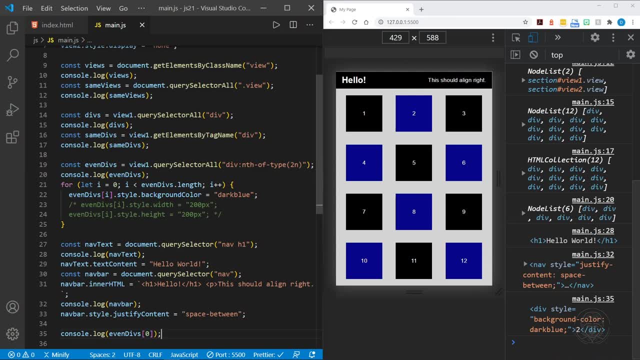 And we're selecting it just like we would select an element in an array. So you can see, there we have a div and the style is background color: dark blue. We set that style and it has the number two in it for text content. 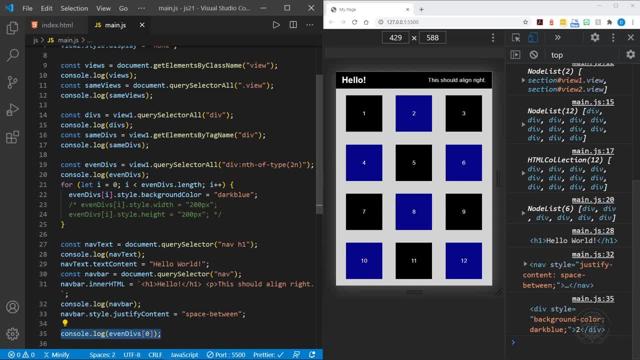 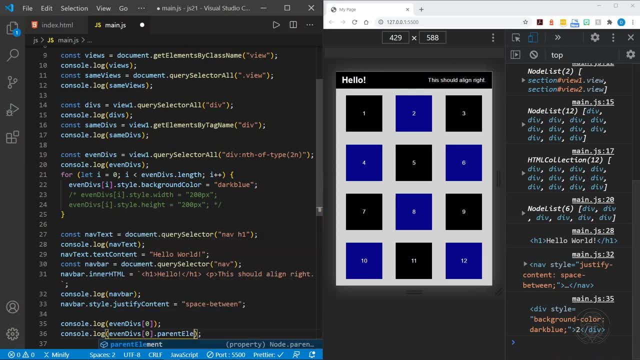 Now this next version, and I'm just going to highlight this copy and paste And the next version. we're going to log the parent element. Using that property, we can see what the parent element of our even div is. And now you see the parent element. 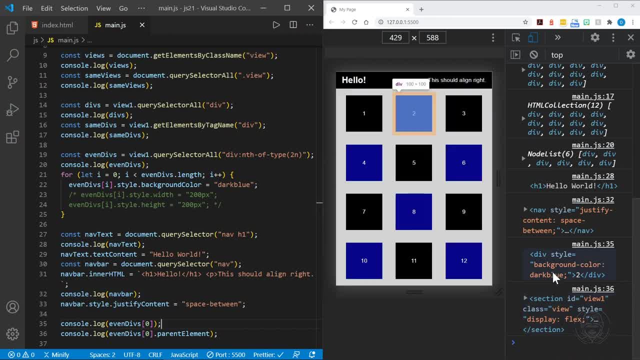 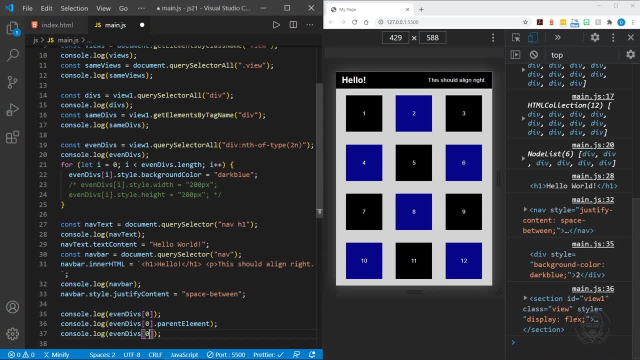 is the full section itself, It is the parent element of this div And we can also say: pardon me, we can also say parent element, So that, once again, is the section, And then we can say: children, Let's see all the children of that parent element. 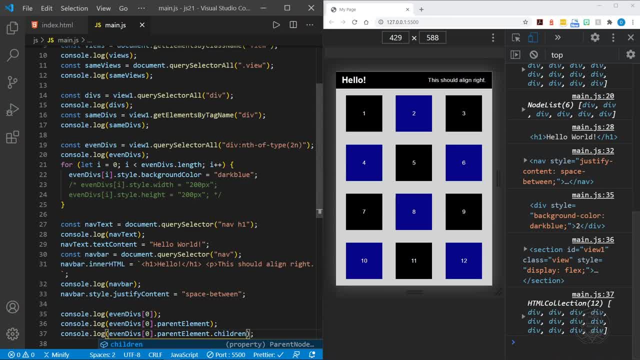 And we get the full HTML collection of 12 divs. Those are all the children of the parent element, And the parent element is the section. So we've navigated from knowing what one div is to finding the parent element, And now we're selecting all of the children. 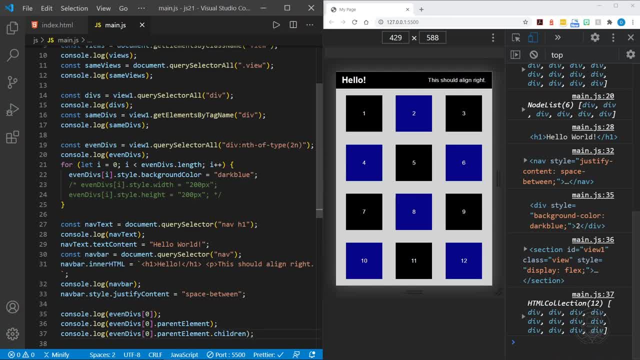 or actually, here we're displaying in the console all of the children. But this is a way to navigate the DOM tree And you can think of the DOM as a tree because you start out with HTML is the main element And, of course, from there, 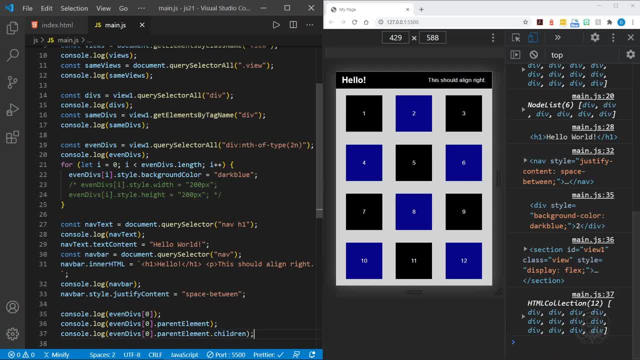 it goes down to usually have a head element and a body element, So those would be the children of HTML, And then they also have their own children And that navigates out kind of like. you see the roots of a tree. So many times it's referred to as the DOM tree. 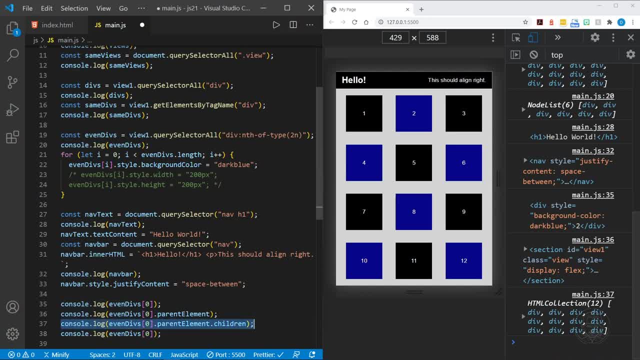 So besides children, let me go ahead and I'm going to use this a few times- So besides just children, if I can highlight this and change it, we can refer to some other properties here. once we get to the parent element, We can say child nodes. 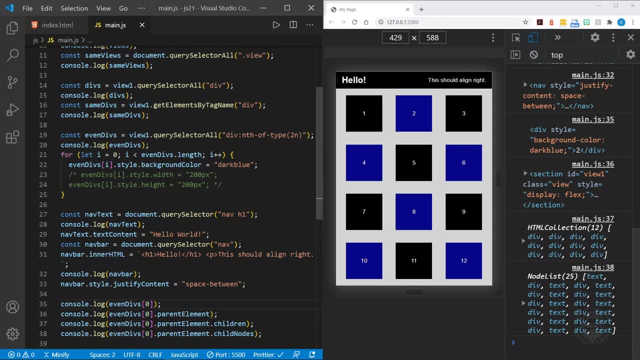 Instead of an HTML collection, like we got with children, we got 25 child nodes. Now what's the difference? The children are actual elements. The child nodes, they aren't just elements. They are elements and also text nodes, Also any white space nodes. 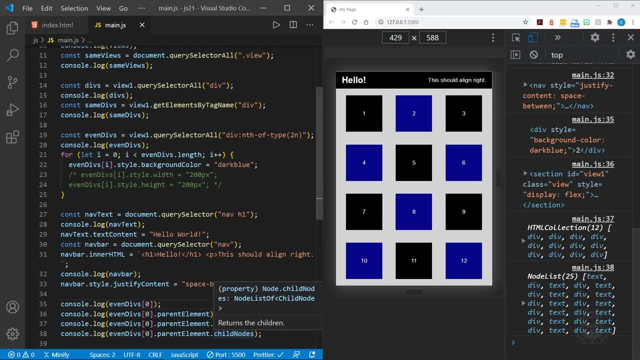 or anything else that might exist. We could easily guess that at least they're double, because we have 12 elements and we have 12 text nodes, And we probably have 12 text nodes. We probably have maybe one extra text node, and that's what it looks like. 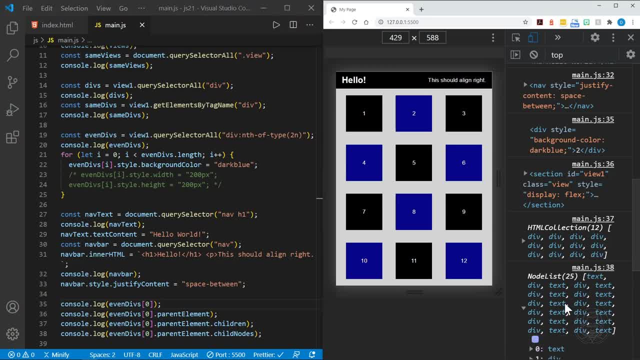 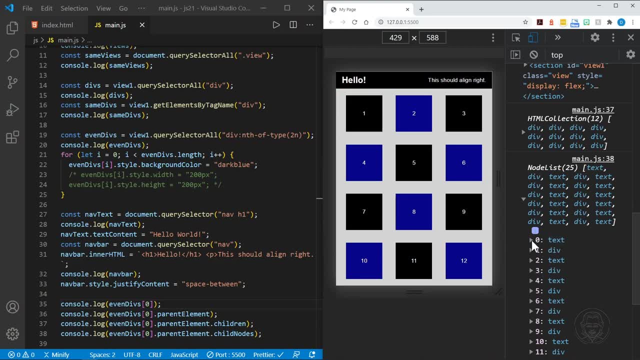 We start off with a text node as well. We could look at each one of these. There's the first div, the next text node, and so on. So let's see what this first text node is. We can look at the text content property. 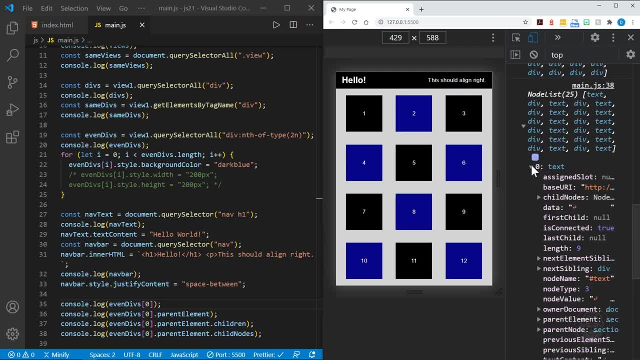 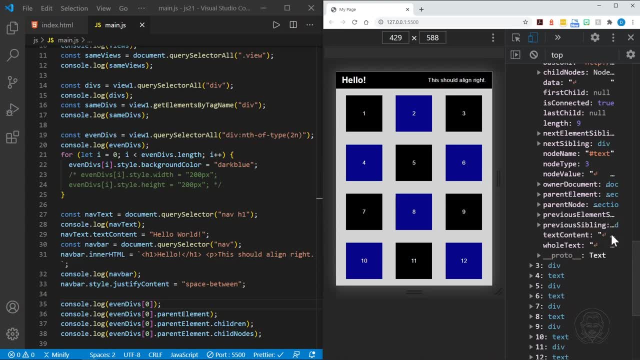 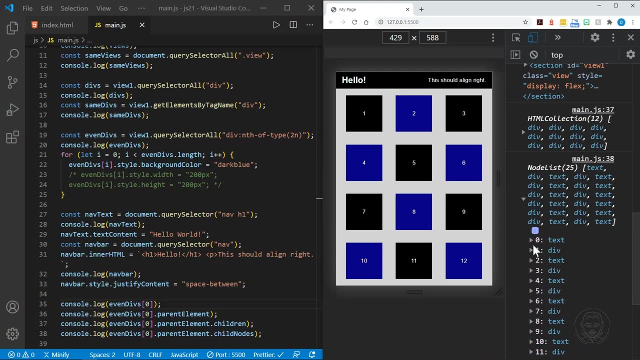 and it looks like it's just a return. So you can see that each one of these- well, it might not just be a return. Can I break that out? Let me see it? Thought, maybe I could open it up. You can see they have all those different properties. 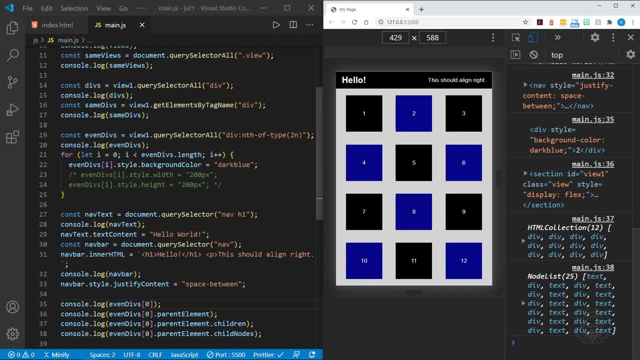 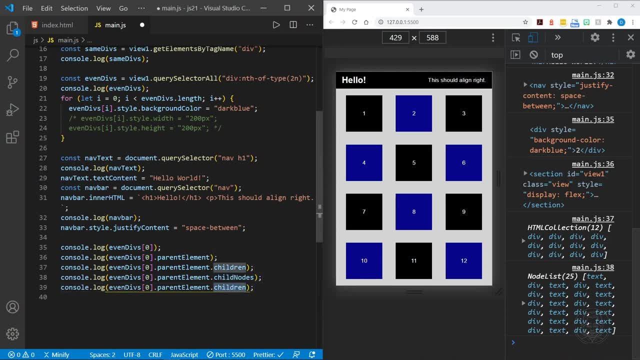 So we have 25 nodes, whereas we only have 12 elements in the same spot. Okay, besides child nodes, we can actually check an element to see if it has child nodes with this method. So has child nodes, save that And it returns 12.. 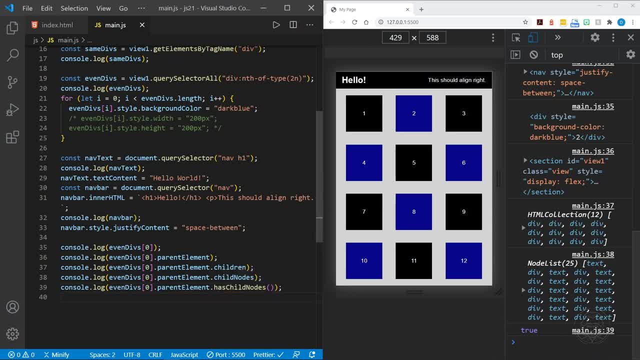 That's true because, yes, it has 25 child nodes. So we knew that was true, but it was worth checking. We could also just pull up the last child And you can see. that is a text node, That is not an element. 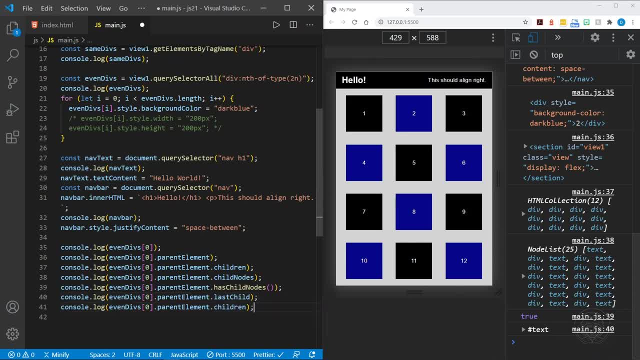 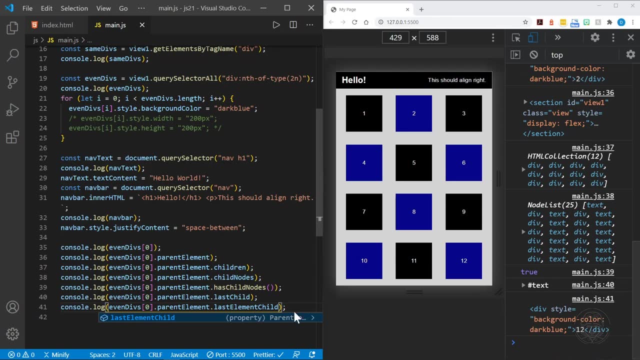 That is the last child of the parent element And you might guess we could also do last element child And that pulls up the very last element of the parent element. And, of course, since there's last child, there's first child There is. 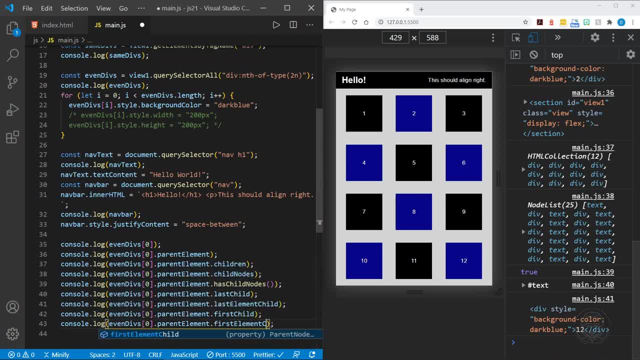 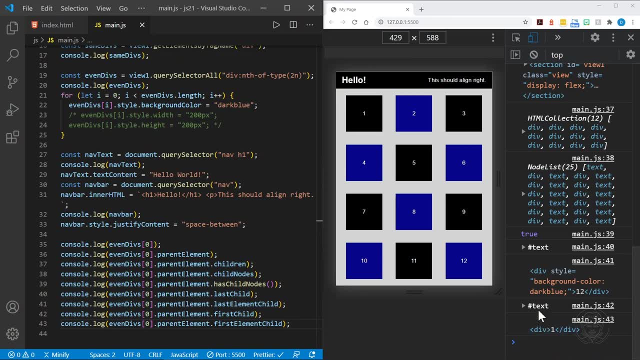 did that wrong. There's first element, child. Save both of those And you can see they are different. The first child is also a text node, But here's our first element, whereas before we pulled up our last element And we could also just get a convenient. 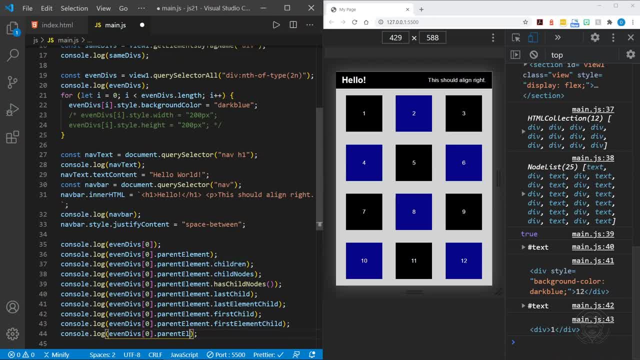 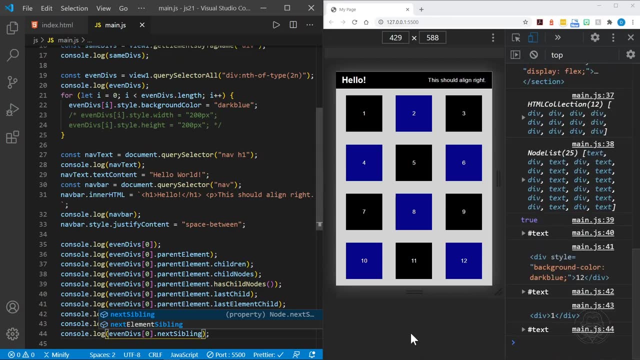 well, let's get rid of the parent element at this point And we're up there, at the very first even element. We're back at number two And let's just select the next sibling. This is a node And you can see the text there. 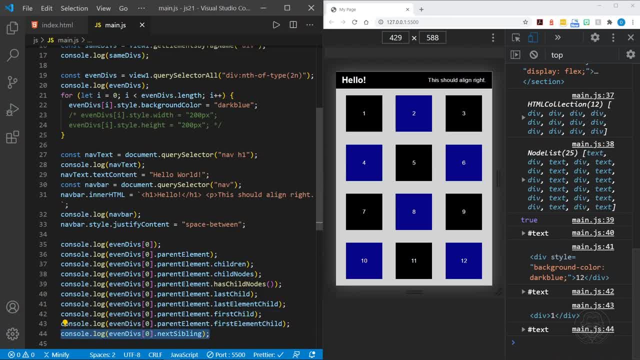 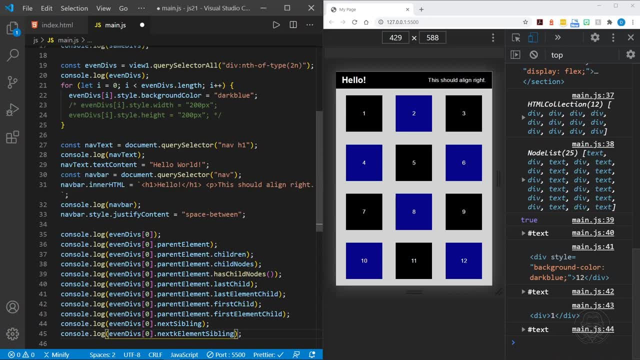 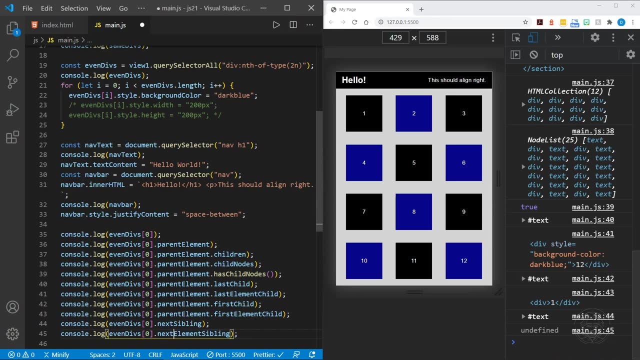 However, you can see the pattern I'm going for here. We could also pull up the next element: sibling. We wanna get to the next element, Ooh, and that says it's undefined, because I put a K in there by a little typo. 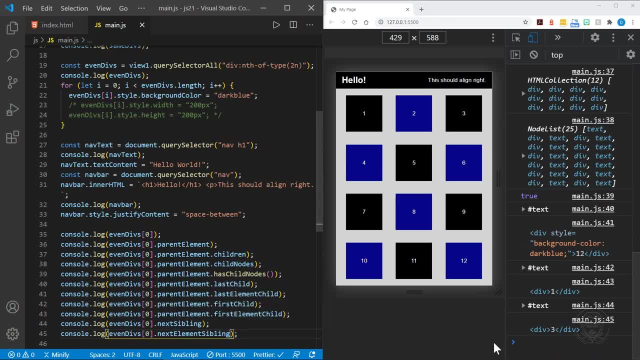 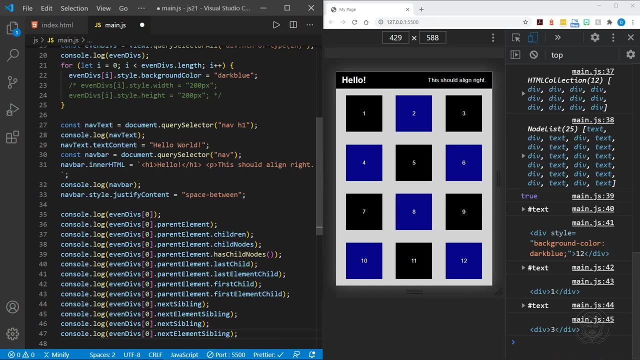 There we go, There's the next element, sibling- And notice that is not an odd one. We had an odd. This went to the very next element. So now it selects number three And of course, with next element, and next sibling, and next element, sibling. 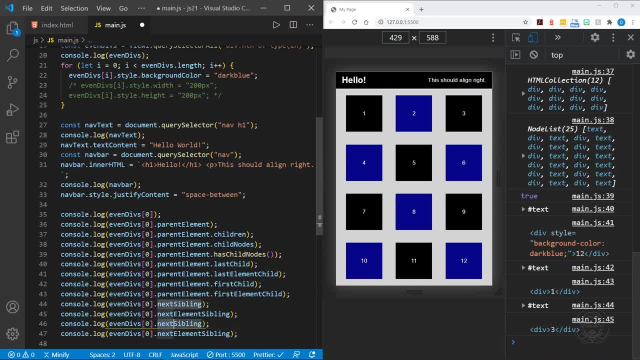 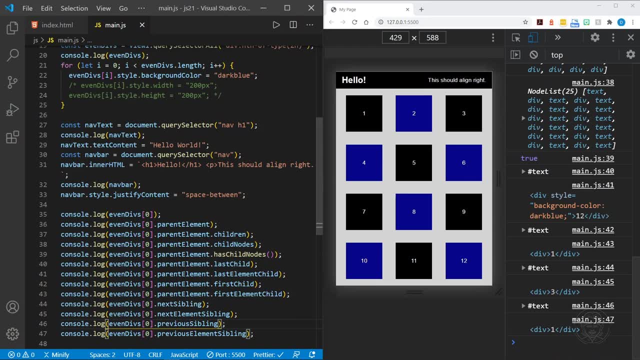 we could also change next to previous And we get both of those as well. So now we got from number three. previous It's still a text node, But now it's number one, And that is a way to navigate the DOM. 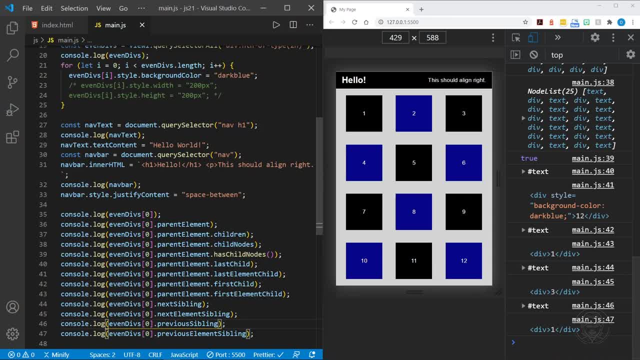 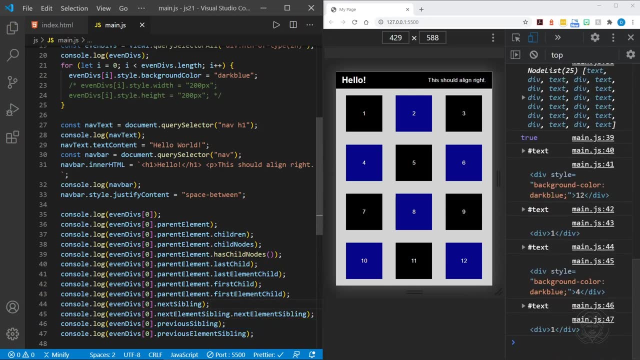 So you could go crazy with this. Actually, you could choose next sibling or next element sibling and then chain another next element sibling and get different results. And you can chain all of these together with dot notation, So you can navigate the DOM in this manner. 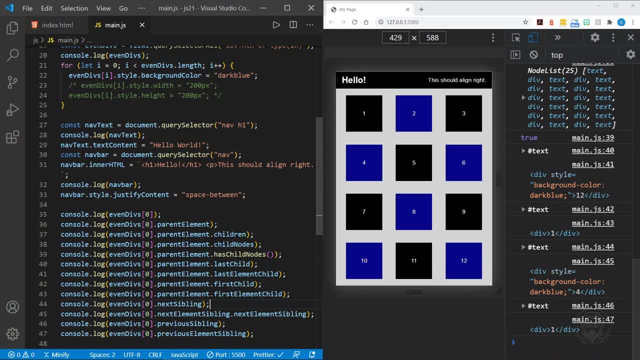 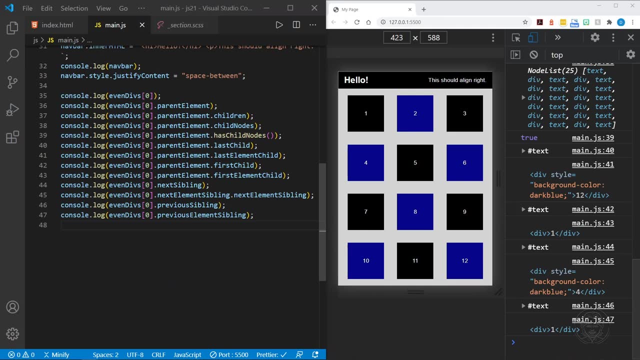 And of course you try not to make it too complicated, But if you need to, you can certainly essentially crawl the page through these different nodes or elements as you navigate the DOM tree. Before we finish, we need to discuss adding to and taking away. 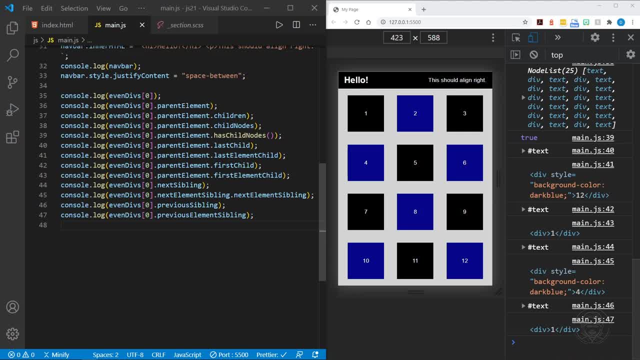 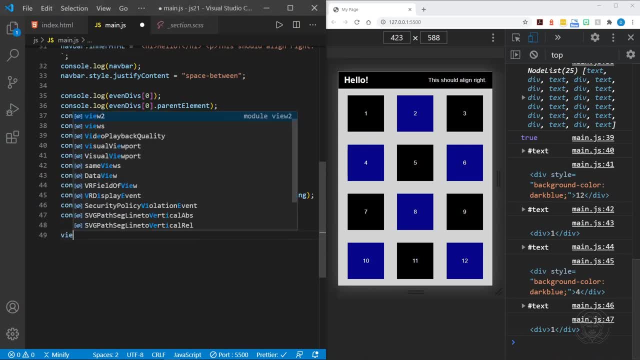 or removing from the DOM. We can create new elements that didn't exist and we can remove elements from the page. Let's make a few tweaks here as we go and we'll check into adding and removing, The first thing we're going to do. 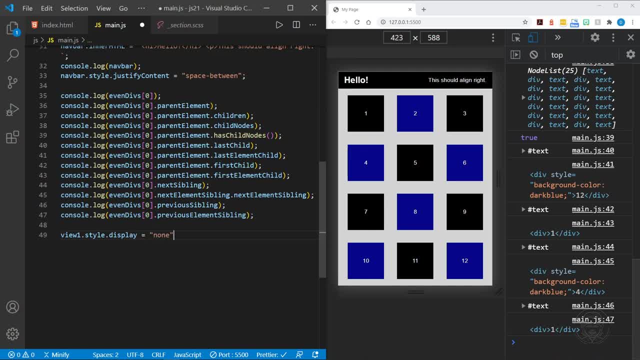 is: hide our first view, our view one. So we'll set that display to none And we're going to show our second view. So we'll set that display equal to flex And we'll save that so you can see that in action. 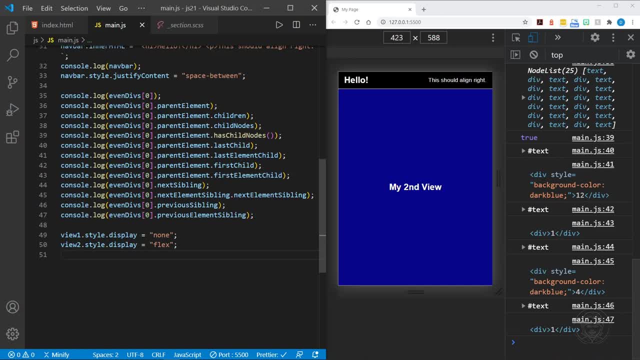 And now the second view is the view that is showing- And now we will take view two and add a couple of more styles to it- that it needs. It needs a flex direction, And we're going to set that to row now instead of column, where it has essentially been at. 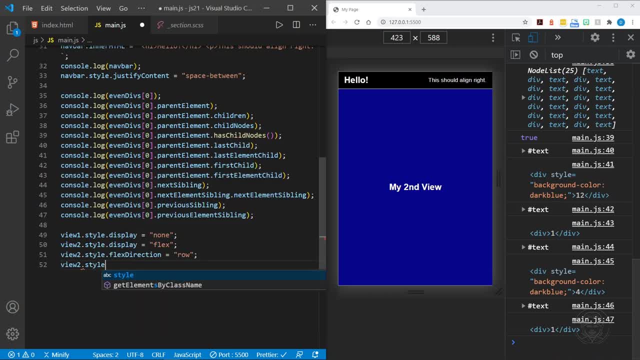 And we're also going to set the flex wrap style. And notice, none of these styles have hyphens like they would in CSS. They go to camel case in JavaScript. So you need to remember that You cannot refer to the hyphenated styles. 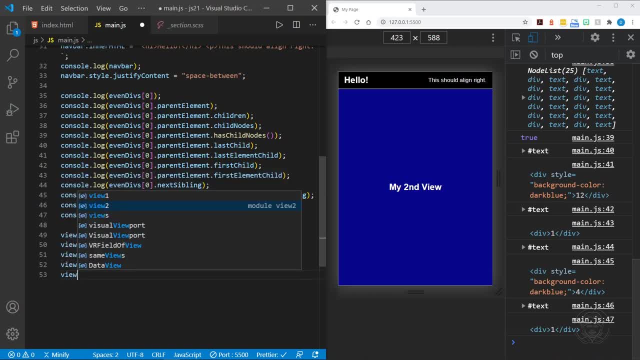 in the same way that you would in CSS, Setting that to wrap. And one more: We've got style And we're going to set the margin equal to 10px, And that should get us started. Okay, now we really don't need. 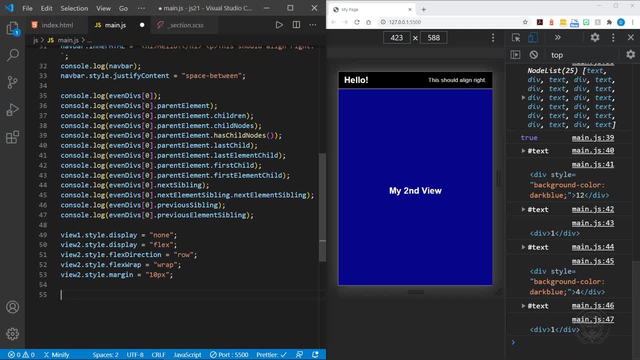 this big. my second view in the middle. And no matter how many elements we have, we can remove those And you can do it rather methodically with a loop. We just need to say view two, last child. So while view two has a last child, 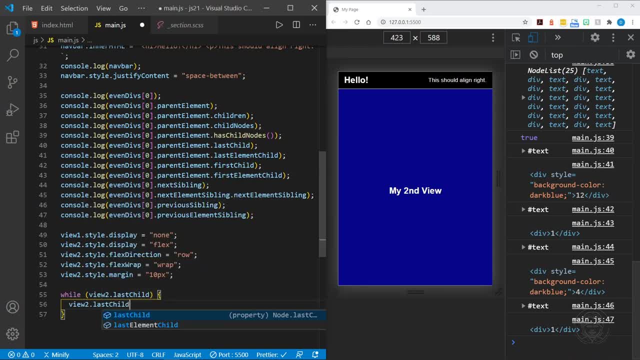 I'm going to refer to the parent here with view two, and then last child and then remove. So we're going to remove all children inside of the view two that we have selected. Now, worth noting here: this is a node we're removing. 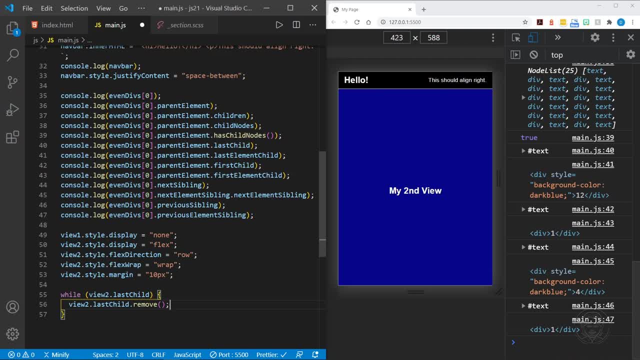 We're not removing just elements, We're removing all nodes, So anything that currently exists inside of this view two, which is a section element itself. So as soon as we save that, our H2 is gone and our second view is entirely empty. 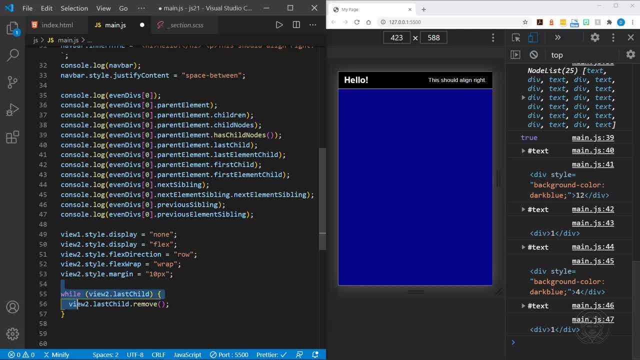 And that comes in useful. So that could be a function you would save and use in an application that is dynamically built, when you need to clear out part of a section or an entire page and then add new content. And right now we're going to add new content. 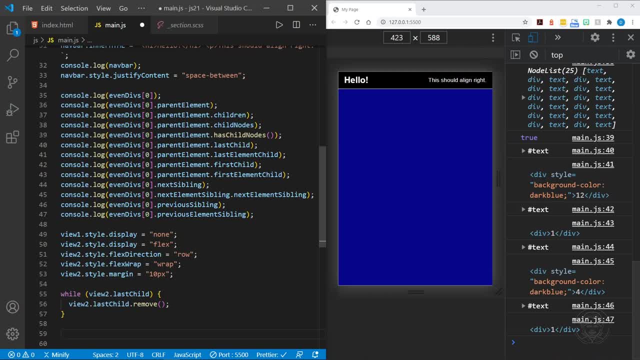 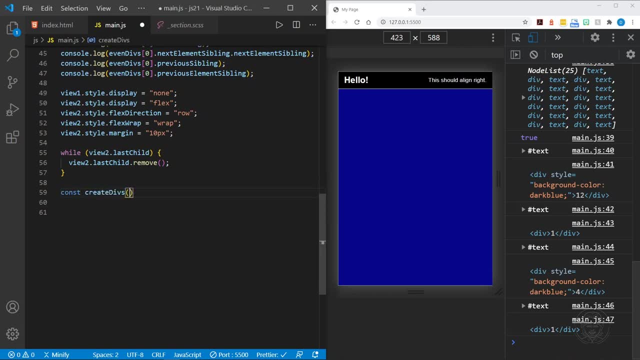 And we should probably make a function when we do that. Let me scroll down and get a little more view here. Let's call this function create divs. Now we're going to feed this function. Well, here, let me go ahead and start with an arrow function. 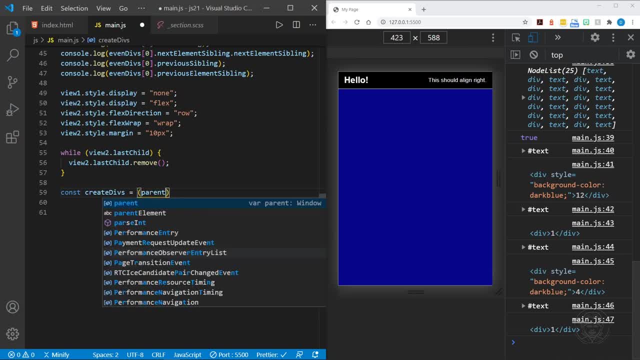 We're going to feed this function a parent element, So I'll just call that parent And we're going to give it an iterator- And I'll show you why in a moment- Because we're really going to put it inside of a loop. 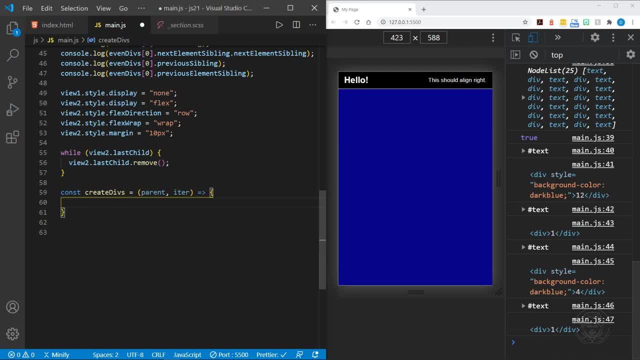 to use this function. So we've got a parent and an iterator. Now, inside the function, we want to create a new div And to do that we're going to use documentcreateElement and specify a div, So that creates a new div element. 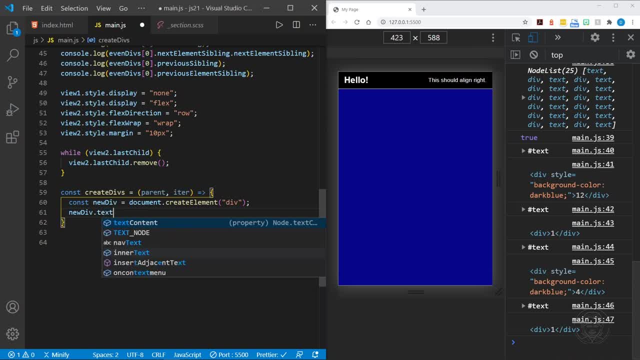 Now we're going to access this new element and add some properties to it. The content itself is going to be the iterator, So we can number each different square we create. The next property we want to access is a style, And we're going to set the background color. 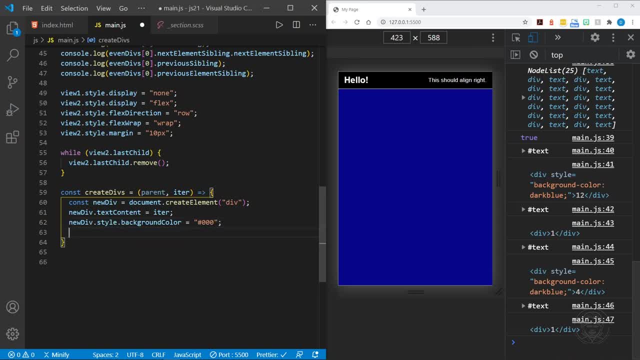 Let's set that equal to black. That is the short notation for black there in the hex notation. The next one, it's going to be the width, And we want to create 100 pixel width, And I should copy this first part so I can paste it. 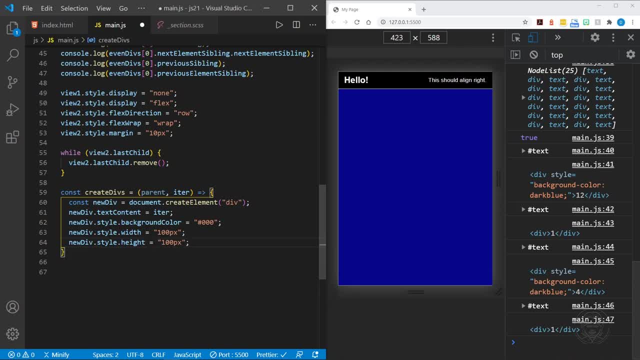 I'm going to paste it each time. 100 pixel height. Go ahead and do that, because we're going to add just a few more. The next one we want to add is margin. We'll add 10 pixels margin to each square. 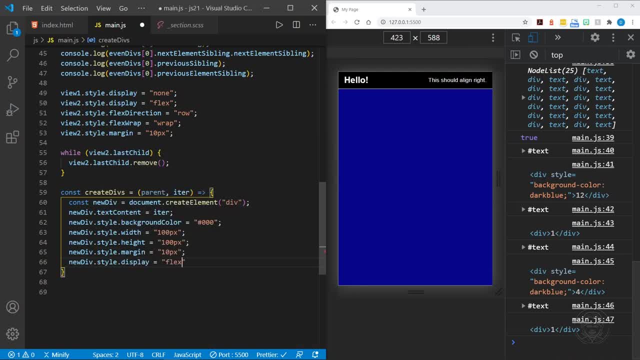 After that, let's set the display of the squares themselves to flex And let's justify that content. And we'll set that to center because we want the number, want the numbers in the center. and now we'll align the items in the center and 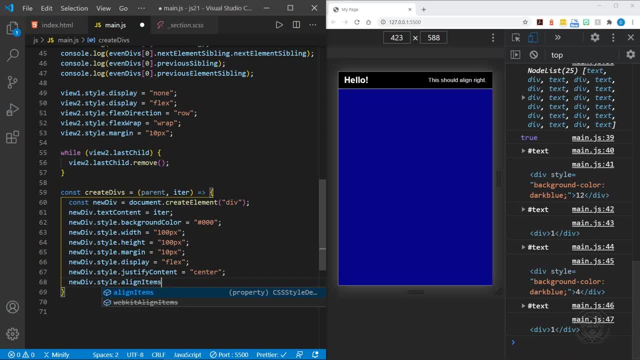 this is more the more what we're centering vertically and horizontally here, and this is the vertical alignment, so Center, and then we need the parent element to append the new element to. so we have our section element that is, view to. that's what we'll end up using, but we're just referring to it because we're 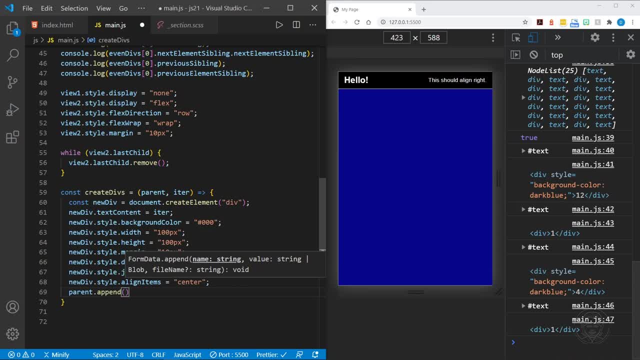 within the function. so we refer to it as the parameter parent and we're going to append the new div we've just created. and there is our function. so let's try that out just one time. so we'll go create divs and we're going to send in. 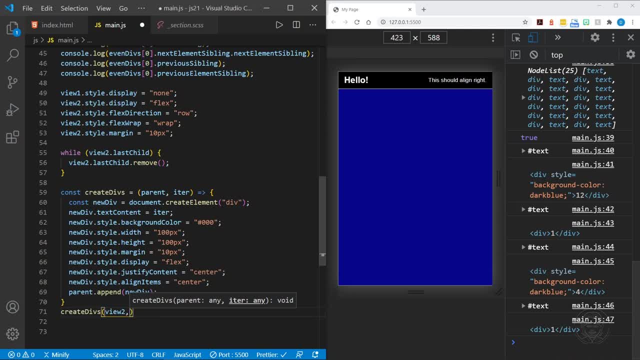 the view to as the parent. and then for an iterator, let's just put in a number. so we'll put in 10 and let's save all of that. and yep, there, we've got one div created and it's centered right in the middle of. 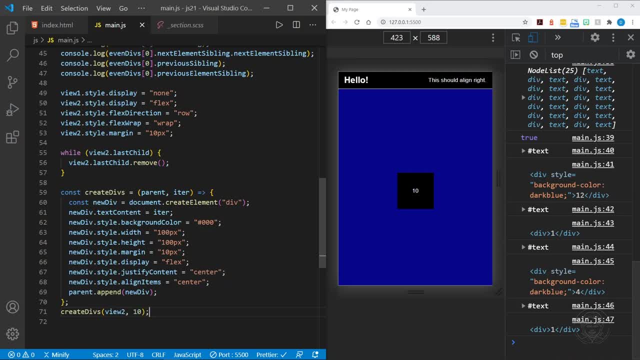 the page as well, and then within that div our number is centered. so not only did our flexbox Center horizontally and vertical inside the div, but we've also got that same style applied to the section. so it took the div we created and centered it horizontally and vertically as well. now, when we add more, 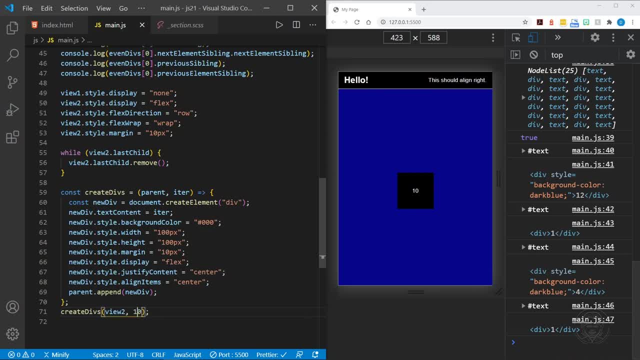 divs, and we can do that through a loop. um um, of course, it will apply the flex styling that we previously saw, in our view, one. so let's create that loop, say for: let I equal and let's start with one, and then, while I is less than or equal to 12, let's increase the iterator. and 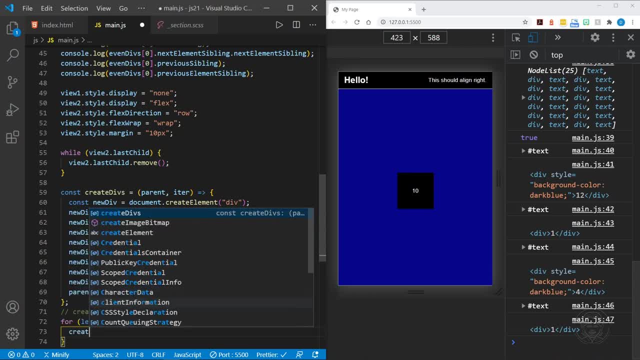 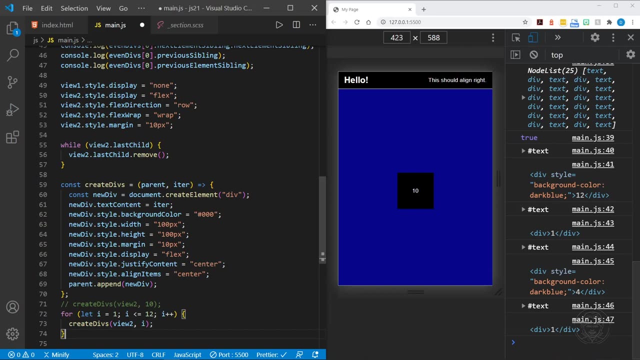 then, inside of our loop, let's call this function, create divs, and we're going to always want to want the new div applied to view two, but then we'll put I in here as our iterator, and that looks pretty good to me. let's save it and see what we get. 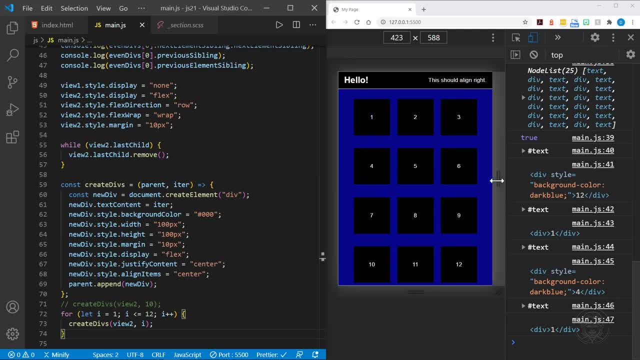 yep, we got 12 divs and it applied the new styling, so it should be a flexbox and respond accordingly, and so that is how you remove, including all divs or nodes or whatever you want to remove. that is a nice little thing you can save as a function to completely clear out a page or a. 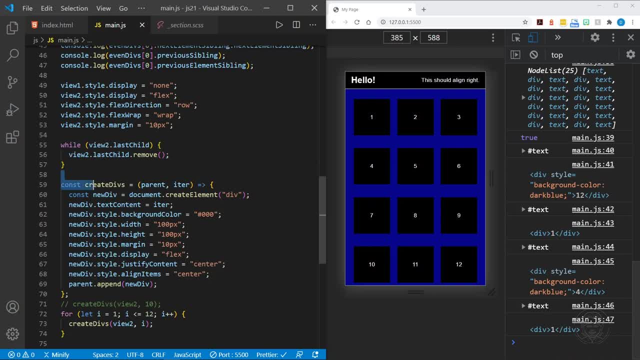 section of a page. and then, with this, you saw not only how we created a new element, we modified many of the properties of the element, and most of those we access- the style property, so we could style it accordingly to our page. and then we appended the new element to its parent element, and that's what made 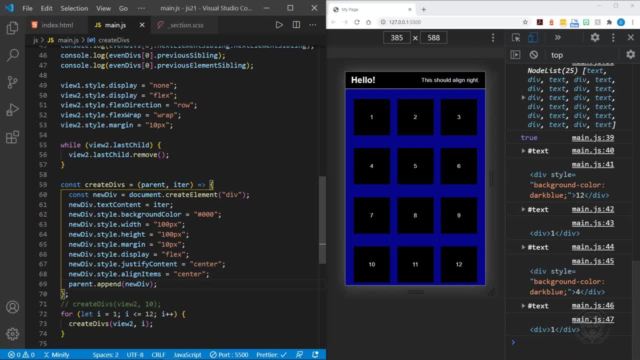 it show up on the page. and then we went ahead and called this function- and it's a function we created within a loop- so we can create 12 new divs and they would be spaced accordingly with the flexbox styling, and that should wrap up this.